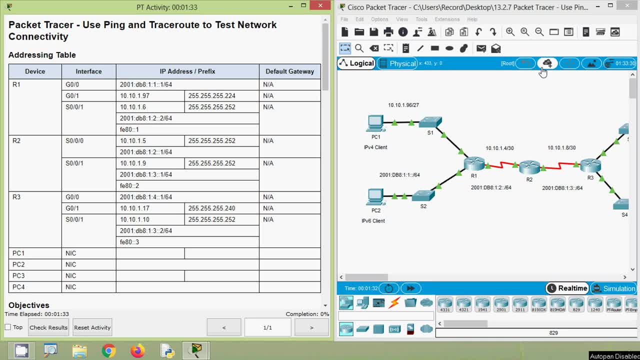 Hi, dear friends, in this video we are going to discuss CCNA version 7 packet tracer activity. Use ping and trace route to test network connectivity. Before coming this activity, friends, if you are watching our channel first time or if you like to get this type of technical videos in future, consider subscribing. 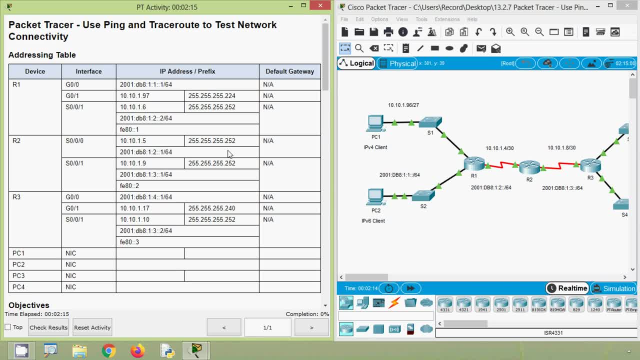 Also, don't forget to enable that bell icon near to the subscribe button so that you will get notification message whenever we upload a new video. And also if you like to get more technical contents or if you like to contact our team, you can visit our website Link I given in the description below. Now back. 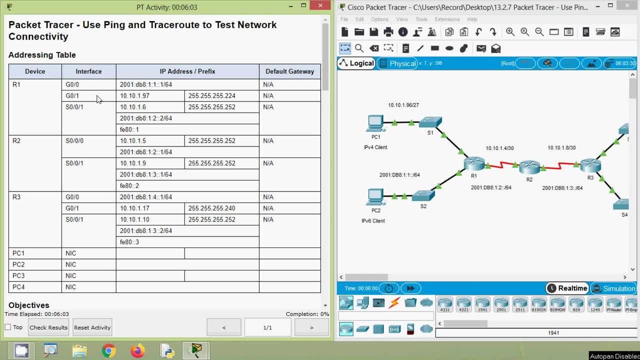 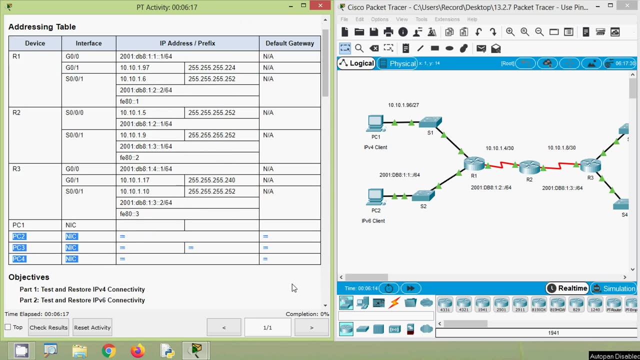 to our activity. Here we can see our addressing table and this addressing table is incomplete. Here we can see PC1, PC2, PC3 and PC4. IP address details are missing. Also, here we can see its default gateway. also we have to update. Here is our. 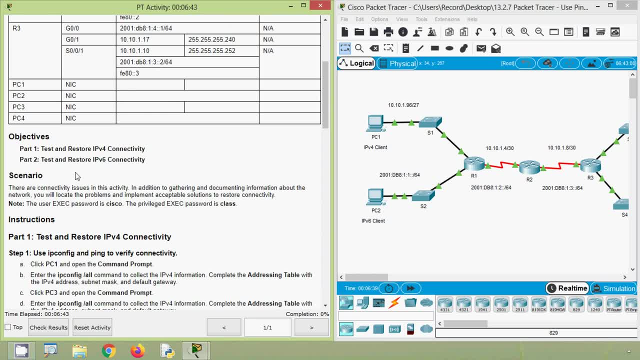 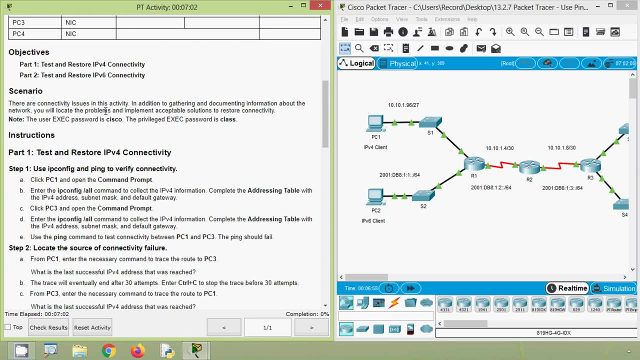 objectives: Test and restore IPv4 connectivity. Also test and restore IPv6 connectivity. There are connectivity issues in this activity. In addition to gathering and documenting information about the network, we will locate the problems and implement acceptable solutions to restore connectivity. Also, the given a note here: the user exit password is Cisco, the privileged exit. 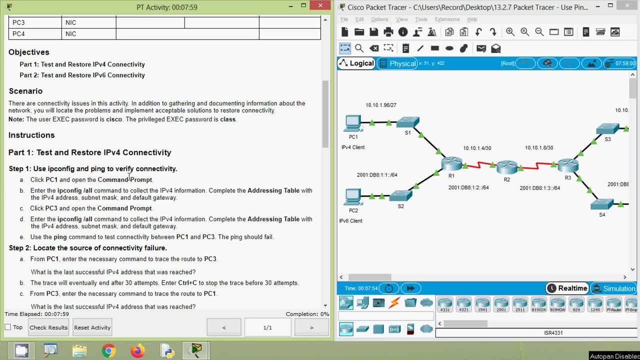 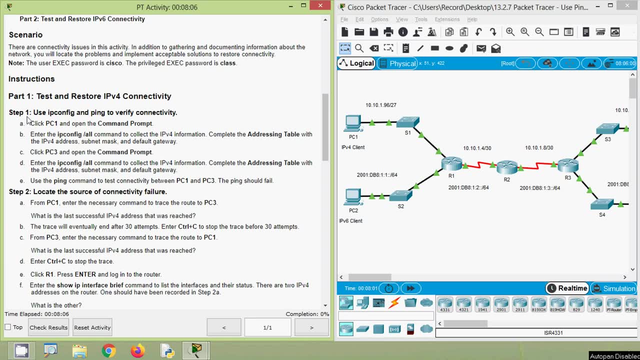 password is class: Okay, Okay, right, so we will go to instructions In part 1, test and restore IPv4 connectivity. Step 1, use IP config and ping to verify connectivity. Click PC1 and open the command prompt. Then enter the IP config. 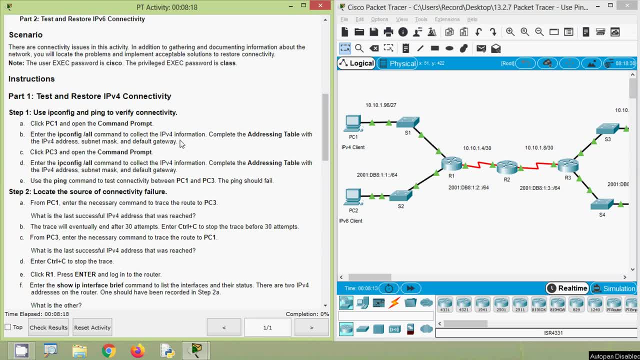 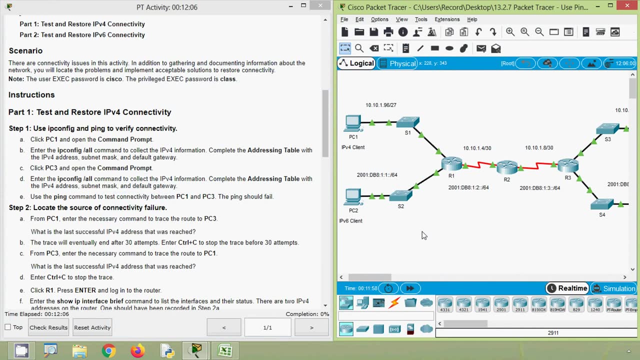 space. slash all command to collect the IPv4 information. Complete the addressing table with the IPv4 address, submit to mask and default gateway. Our addressing table is ready with our spreadsheet, So now we will go to this PC1 and we will check. 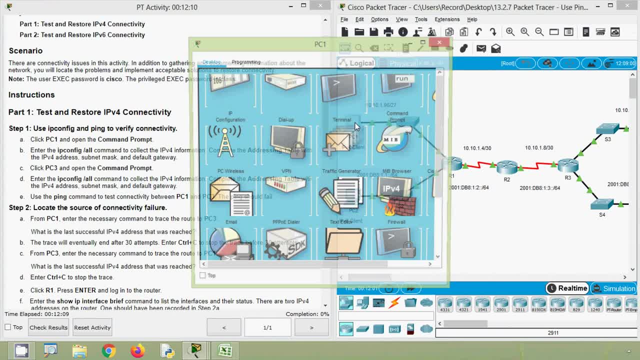 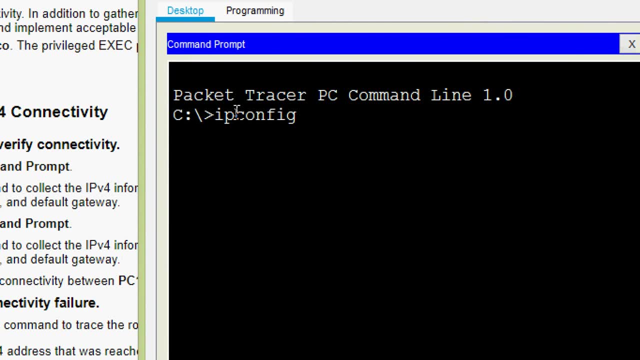 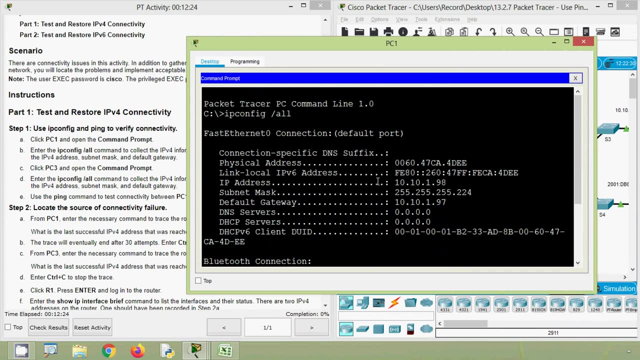 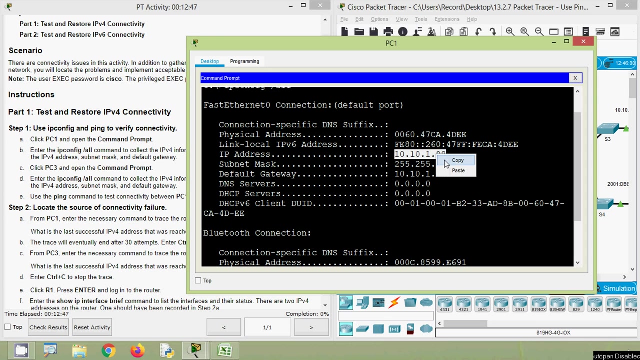 its IPv4 address. So, coming to PC1, we'll go to command prompt and here we will give that command, IP config, space, slash, all, and here we can see the details, Here we can see its IP address. We will copy this IP address. and coming to our 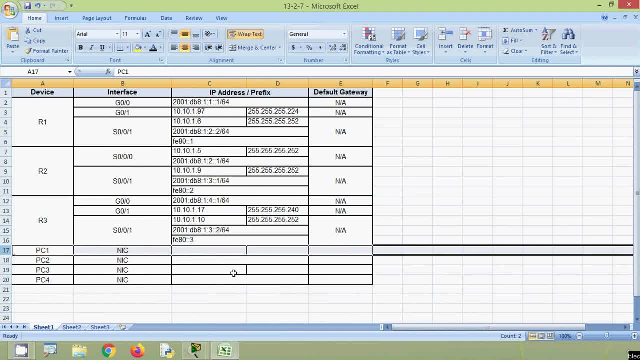 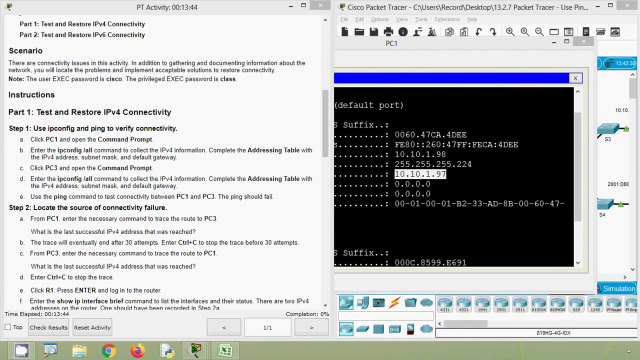 spreadsheet PC1.. Okay, here we will give that. Then we have to give its submit to mask. Okay, then its default gateway. We'll copy that. Okay, right Now. click PC3 and open the command prompt. Then enter the same command, IP config space. slash all to collect the IPv4 information, Then complete. 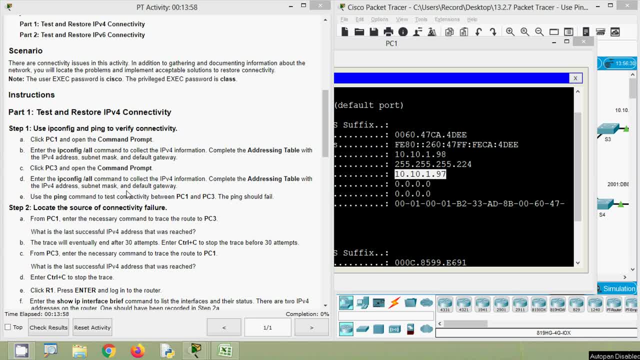 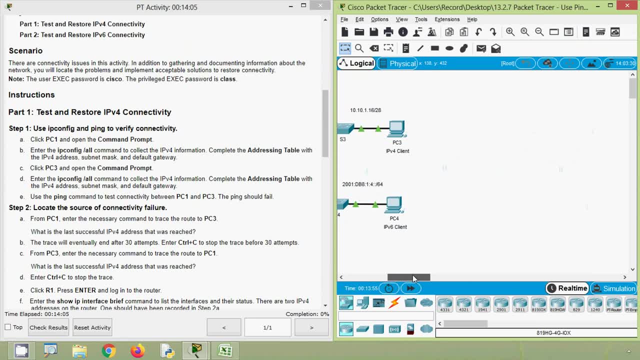 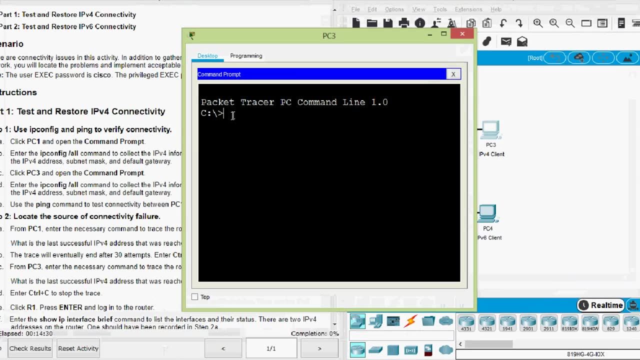 the addressing table with the IPv4 address: submit to mask and its default gateway. Okay, now we will go to PC3.. Sure, we can see our PC3. We will click on it. then, coming to command prompt, Mobil salvation application to the PC prompt mode to: 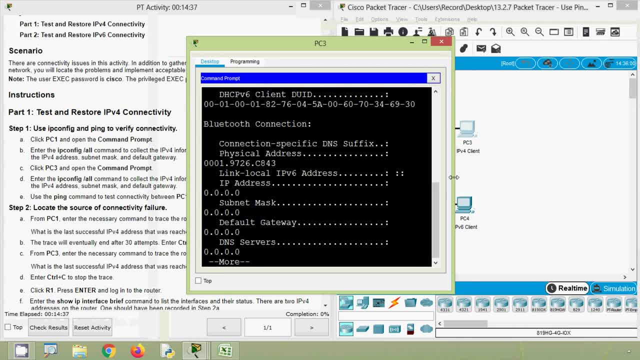 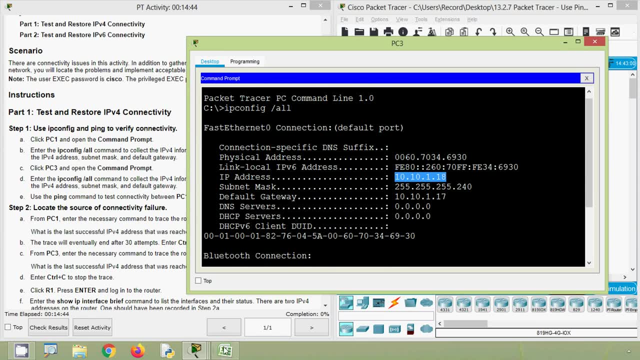 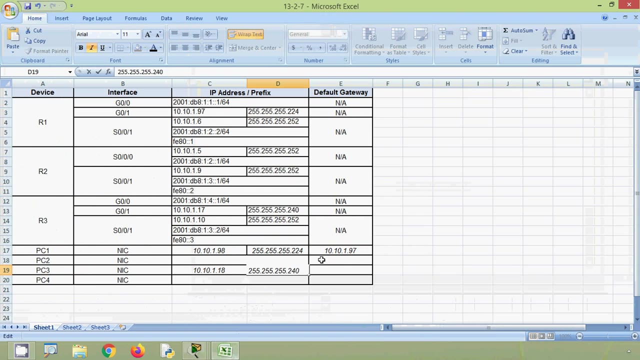 invoke any IPv4 application: ger. we can see its IP address. We will copy this address: PC3, okay, Now we have to get its IP address, Put the excel to the desktop and after that we will Submit mask. Okay, then it's default gateway. 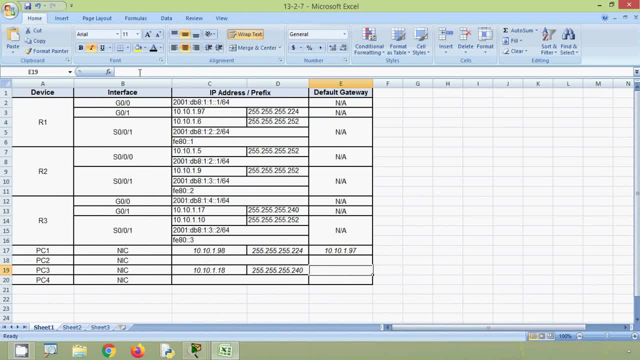 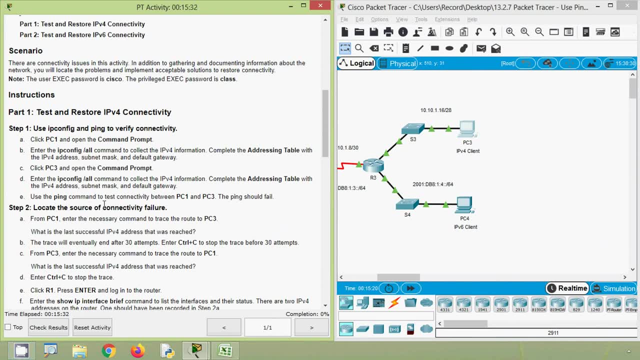 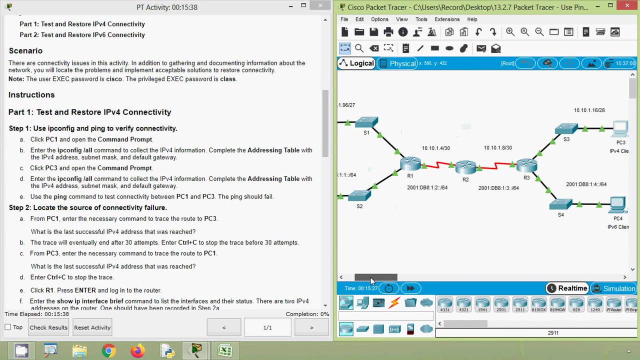 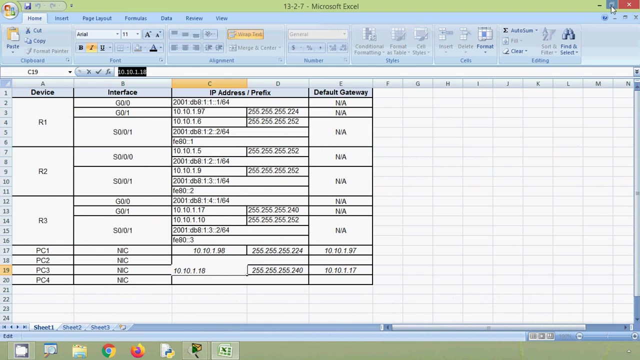 We'll copy it and it's here. Now use the ping command to test connectivity between pc1 and pc3. the ping should fail. Okay, we will do that. So just we will copy PC3 IP address. Then we will go to pc1 command prompt. here we will give that ping. 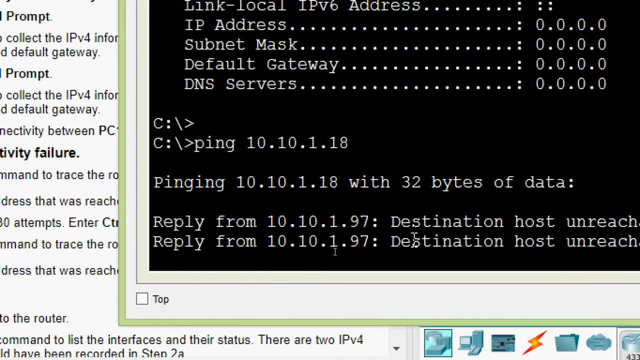 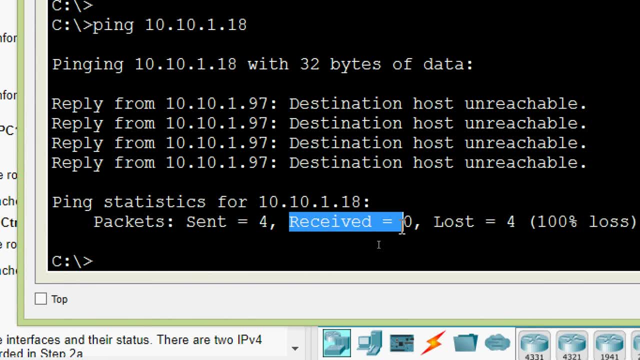 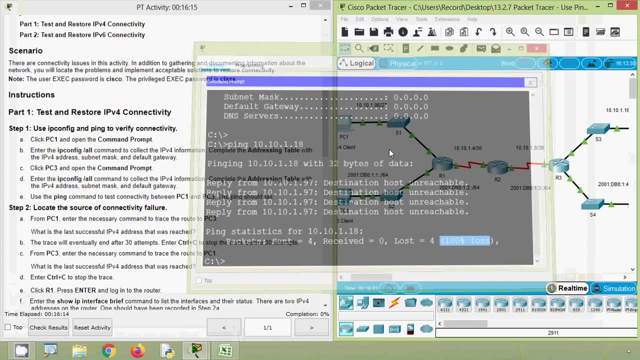 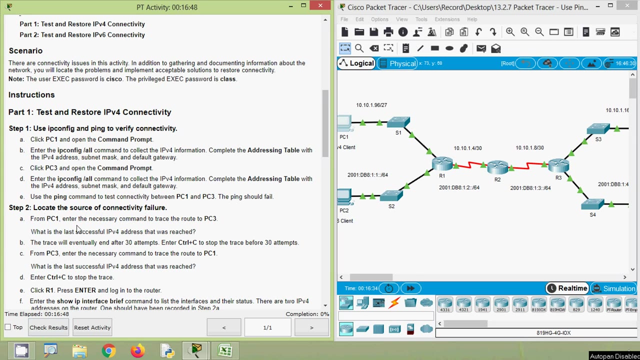 Then pc3 address and Here we get the destination housed Unreachable. so here we can see: packet sent for but received a zero, lost four, 100% a loss. So it's failed. Now coming to step to locate the source of connectivity failure: from pc1, enter the necessary command to trace the route. 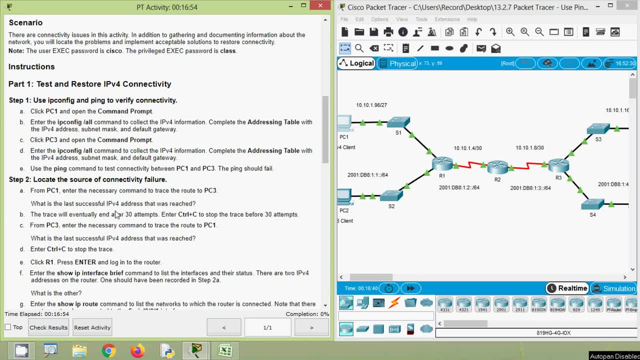 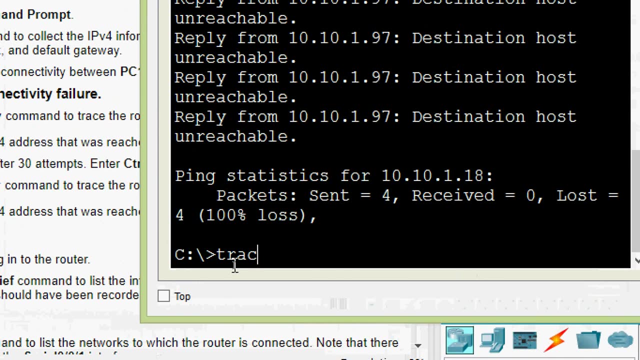 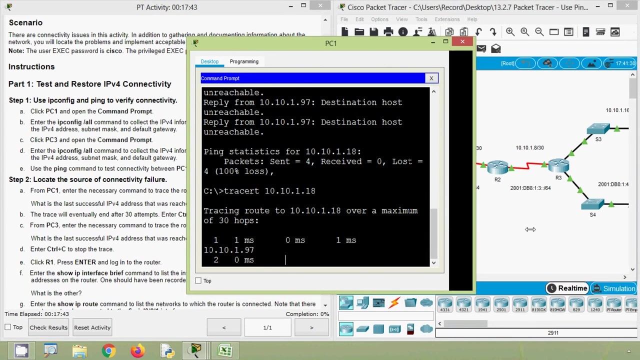 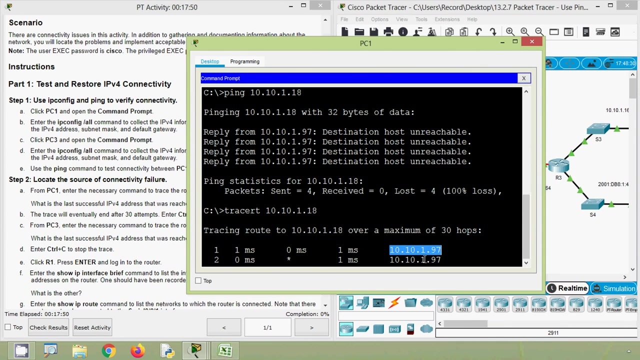 to pc3. What is the last successful IP before address that was reached? Okay, we will give this trace command on pc1. So we will give Tracer to then our pc3 IP address. So here we go: 10 dot 10 dot, 1 dot, 97 and the same address again. 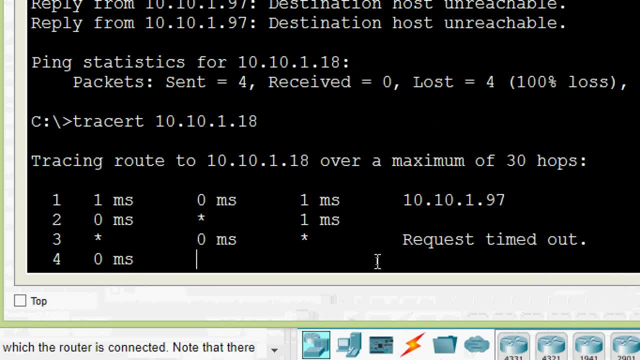 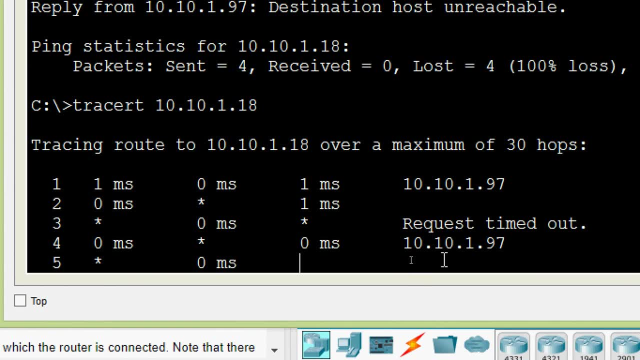 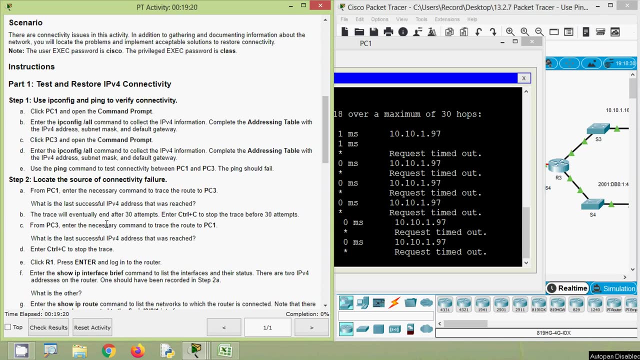 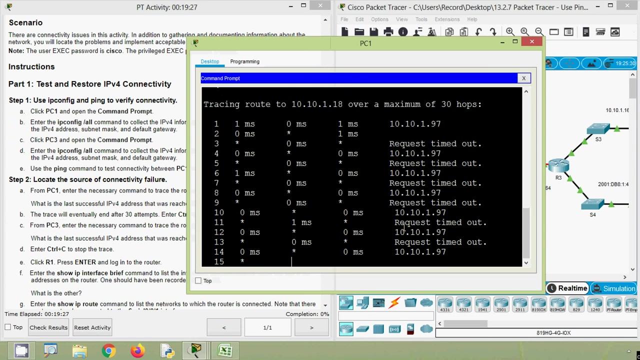 Request time doubt. So here we can see the last IP address we received. It's a 10 dot 10 dot 1 dot 97. Now the trace will eventually end after 30 attempts. enter ctrl C to stop the trace before 30 attempts. Okay, here we get the same IP address again and again. so we can stop it by using this. 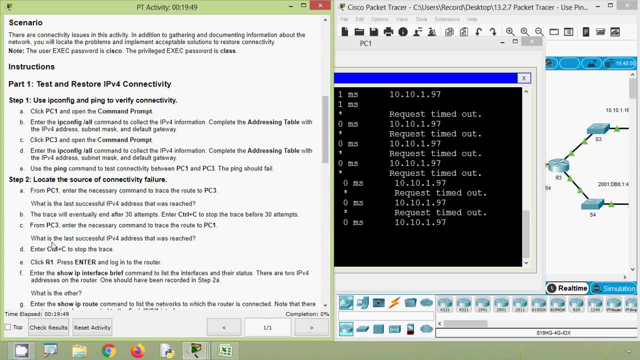 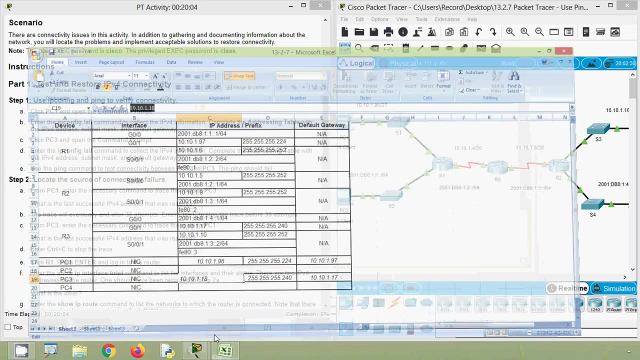 ctrl C Now from pc3, enter the necessary command To trace the route to pc1. and what is the last successful IP before address that was reached? Okay, So first of all we will get our pc1 IP address. Okay, now we will go to. 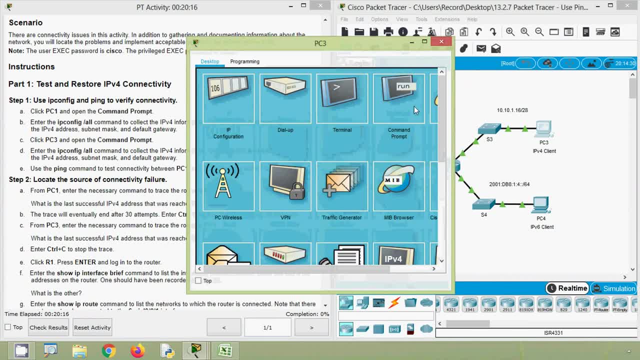 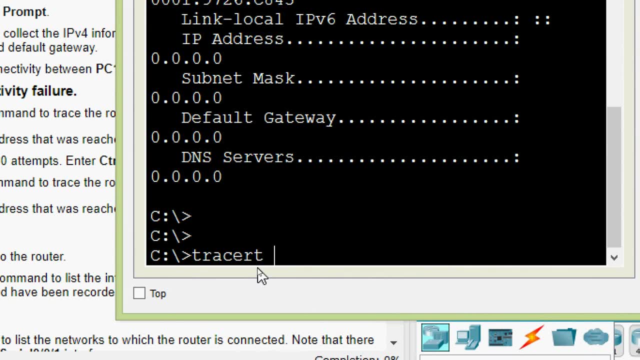 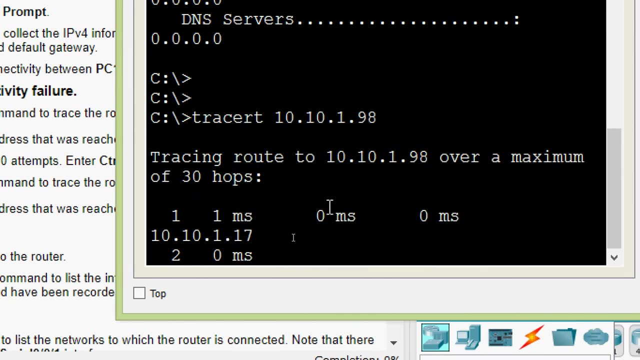 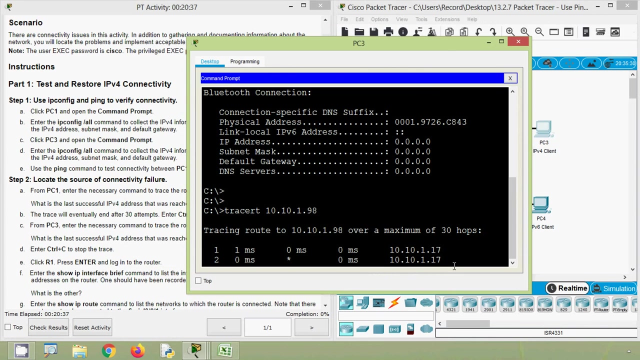 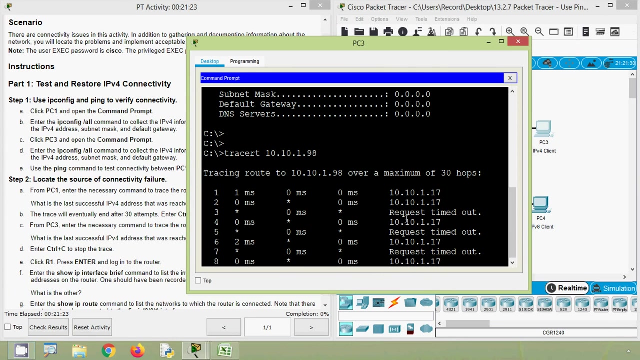 PC3. You will give a trace route command here, Tracer. Here is a pc1 IP address: 10 dot 10 dot 1 dot 17. Now here we can see the last successful IP before address. it's a 10 dot 10 dot 1 dot 17. 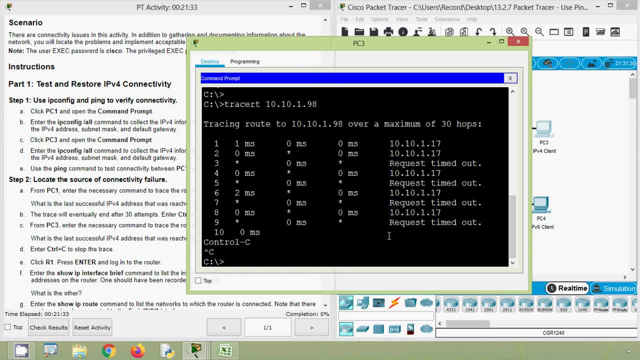 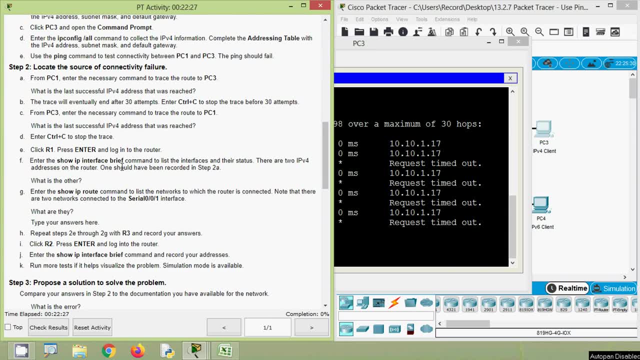 Enter ctrl C to stop the trace. Okay, Now click R1, then press enter and a login into the router. enter the show IP interface brief command to list the interfaces and their status. Enter ctrl C to stop the trace. Now click R1, then press enter and a login into the router. enter the show IP interface brief command to list the interfaces and their status. 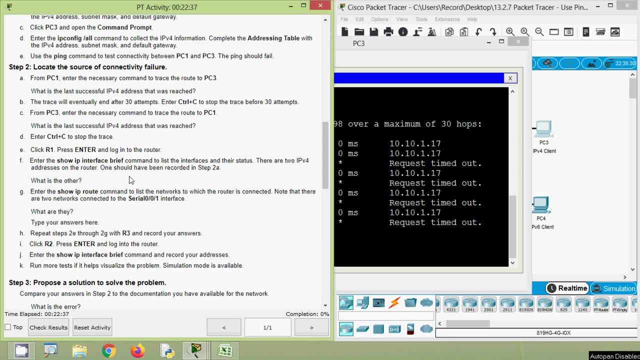 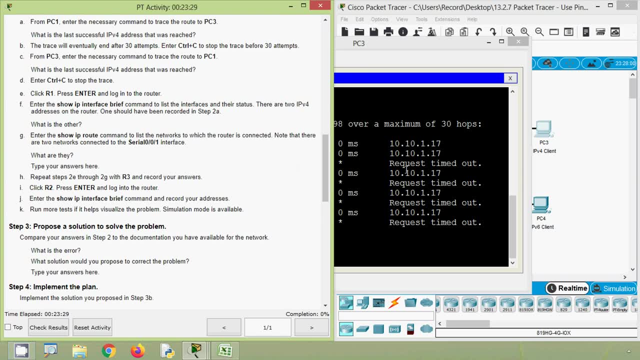 There are two IP before addresses on the router. one should have been a record in step 2a. What is the other? Okay, we can do that. We will close this pc3 and coming to. Okay, we can do that. We will close this pc3 and coming to. 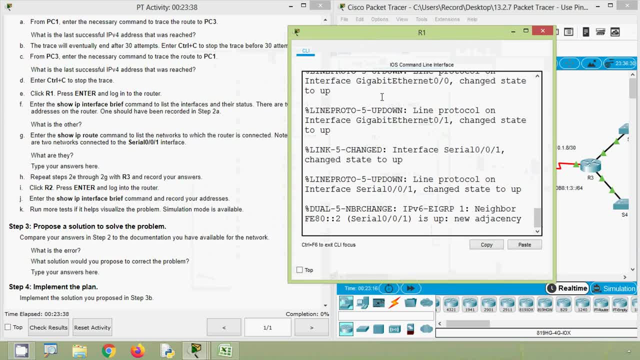 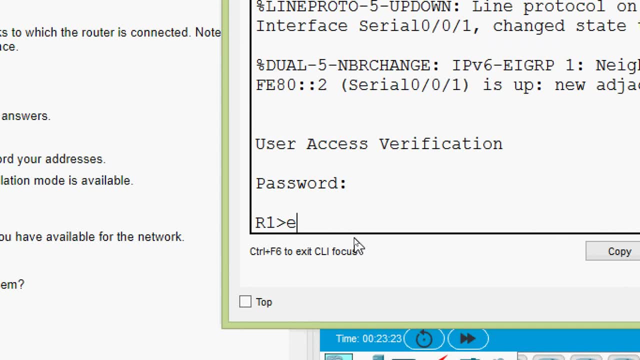 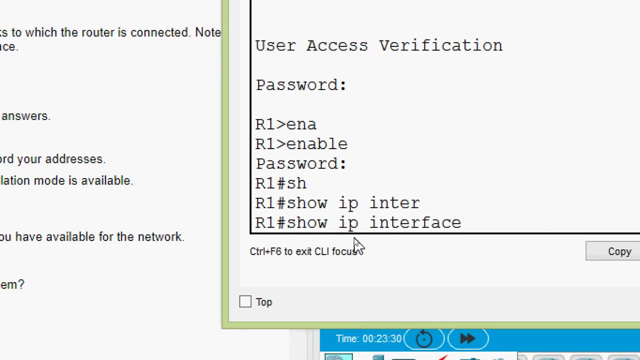 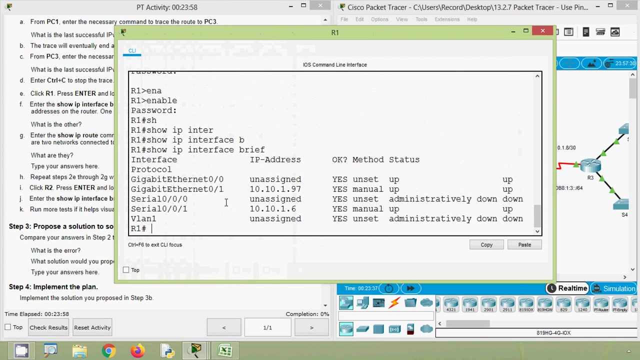 router r1 cli. here we will give that command. so before that user access verification. password is cisco enable. password is class. so here we will give show ip interface brief, and here we can see ip address details. gigabit third, zero slash one: 10.10.1.97. it's status up. 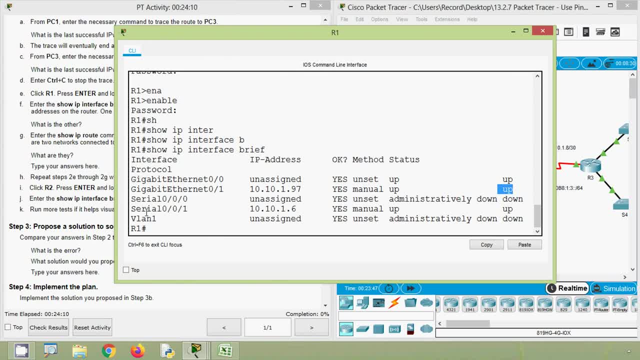 protocol also up and here we can see serial 0.0.1- 10.10.1.6. status up protocol also up. now here we can see the ip address which we got. uh, when we trace from pc1 to pc3, so coming to pc1, and here we can see that. 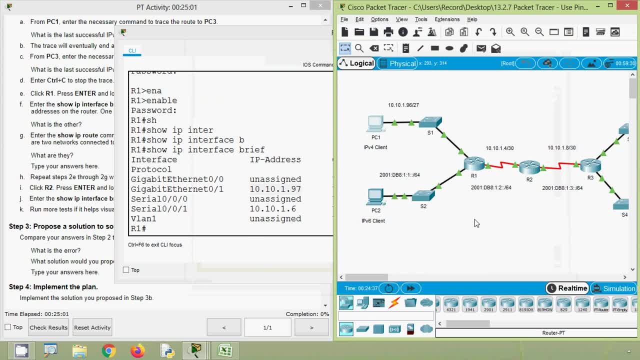 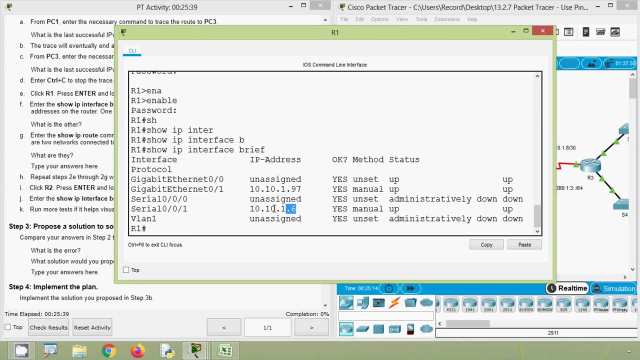 10.10.1.97 the ip address of this interface gigabit threat 0, 1 in this router r1. and now here we can see the other ip address: uh, it's a 10.10.1.6. uh for the interface serial 0, 0, 1. 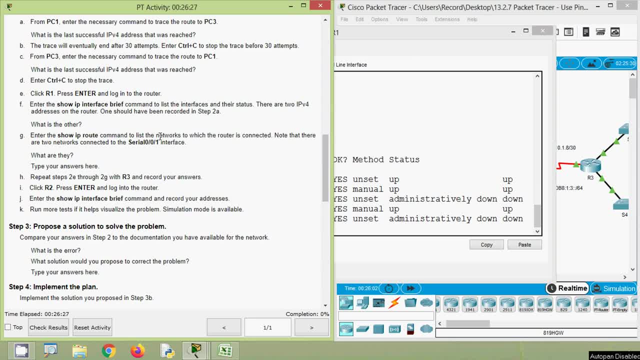 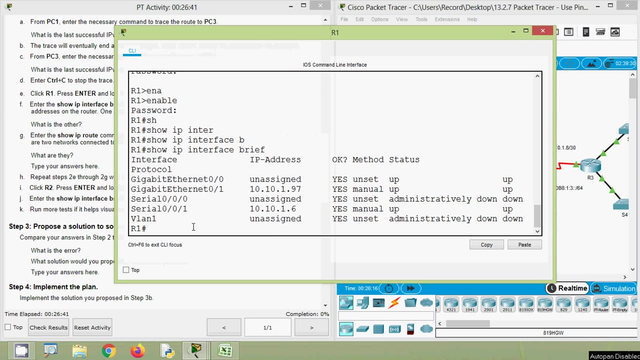 now enter the show ip root command to list the networks to which the router is connected. note that there are two networks connected to the serial 0 0 0 1 interface. what are they? type your answer here: okay, so we will give that command here. 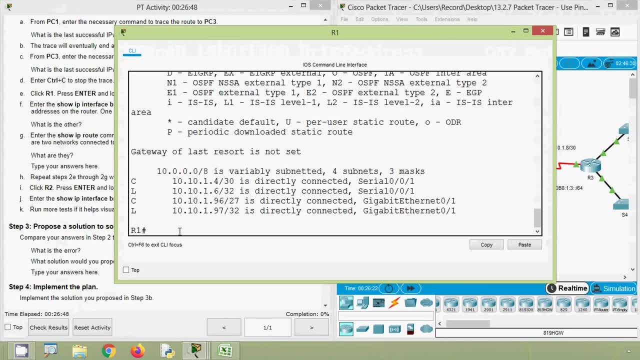 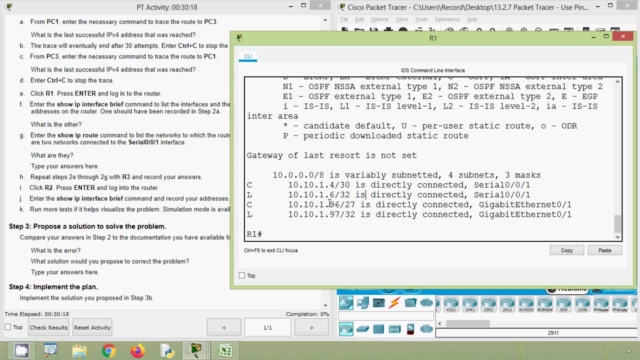 show ip root. yes, now here we can see two networks are connected to the interface: serial 0, slash 0, slash 1. first one connected 10 dot 10 dot 1 dot 4, slash 30 is directly connected to serial 0, slash 0, slash 1. 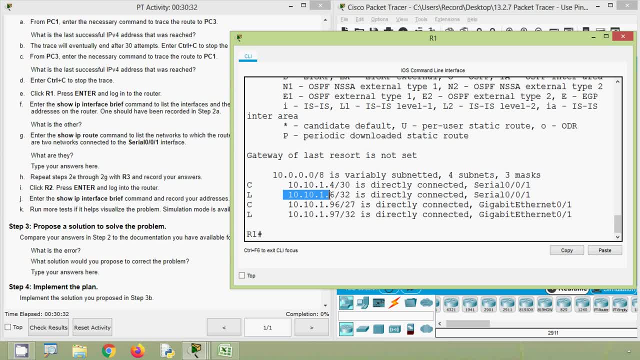 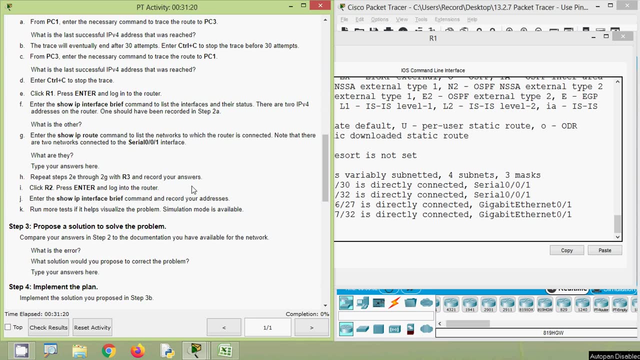 and here we can see a local 10 dot 10 dot 1 dot 6. slash 32 is directly connected. serial 0, slash 0, slash 1. now repeat steps 2e through 2g with r3 and record your answers. okay, we can do that coming. 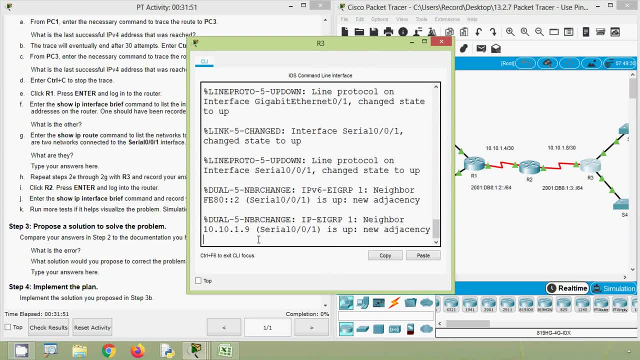 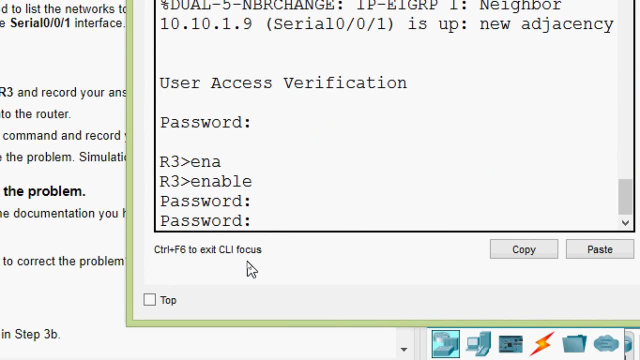 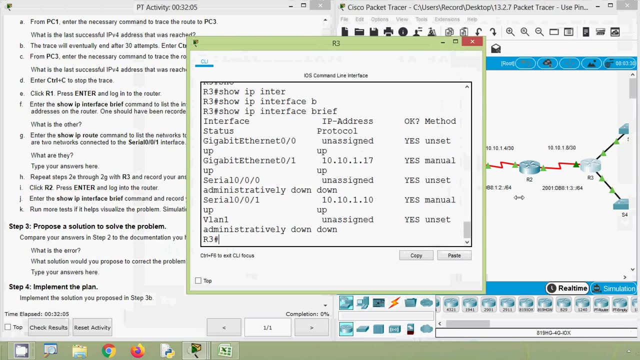 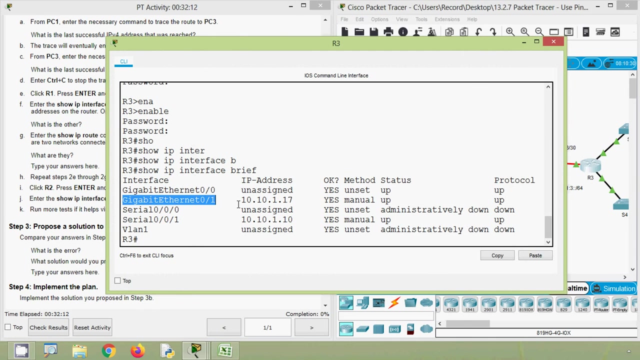 to router r3. we'll go to CLI. password is Cisco enable. password is class. okay, here we are going to give show IP interface brief and here we can see gigabit: a term 0 slash 1. its IP address: 10 dot tendered 1.17 status. 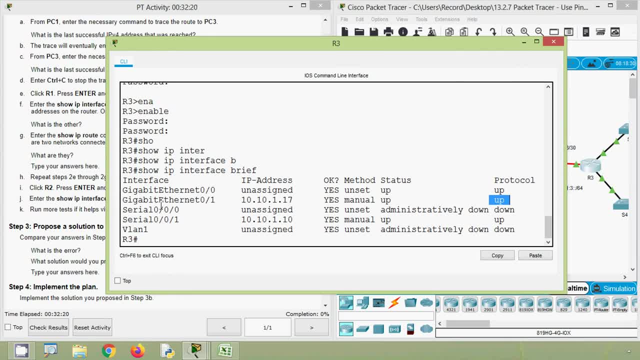 absolutely also also we can see the interface serial 0 slash 0, slash 1. its IP address, 10 dot 10 dot 1 dot 10 status up protocol. also up and during our trays we have seen this IP address or we haveliness, and we can see the Waypoint keypad. we can get the altram ships, thank you. for watching the video to the end, like E feels so much fun. check the rest of the lesson. if you have now watched the video, please don't forget to subscribe to mine and checking the other videos as well. as. לע biotekincom. we will see the right link here, and here is the arabic buenas, and we have. 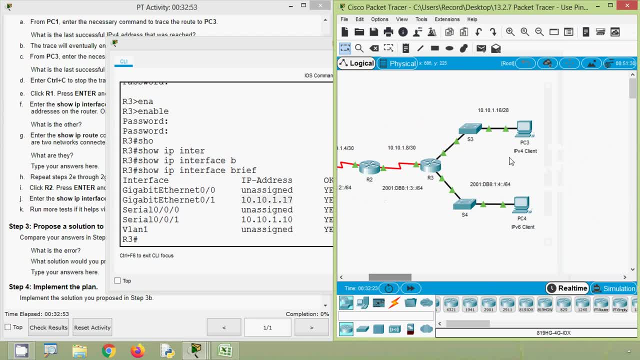 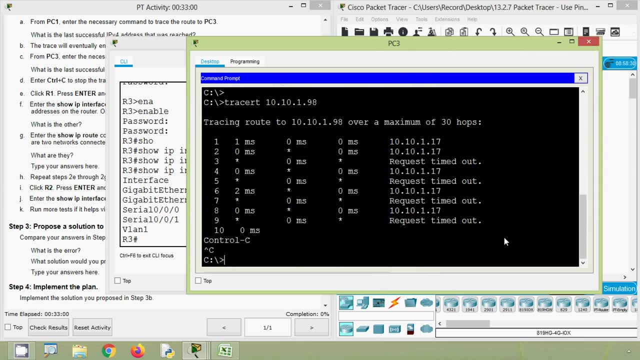 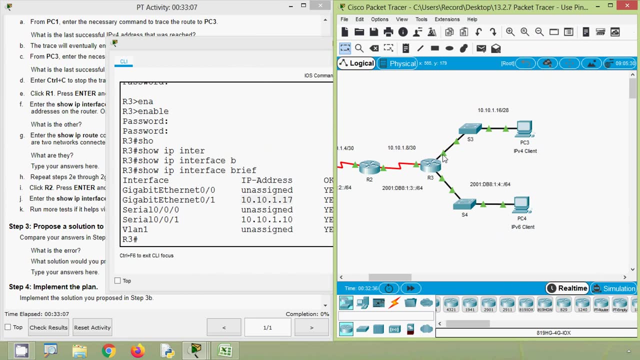 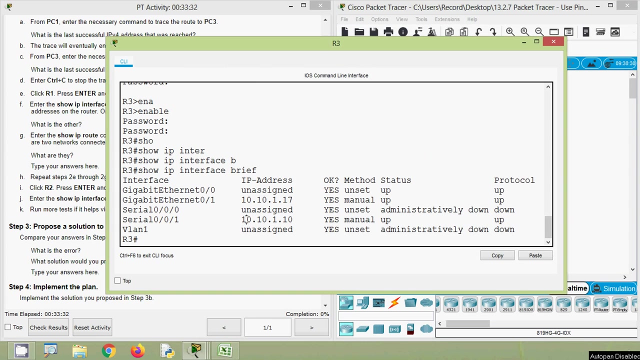 10.10.1.17. so, coming to our pc3 command prompt, here we can see that it's here the ip address of this interface gigabit, third zero slash one in this router r3. so the next address is a 10.10.1.10 for the interface serial. zero slash, zero slash one. 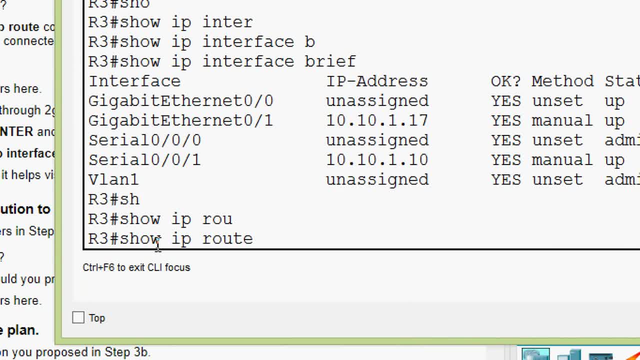 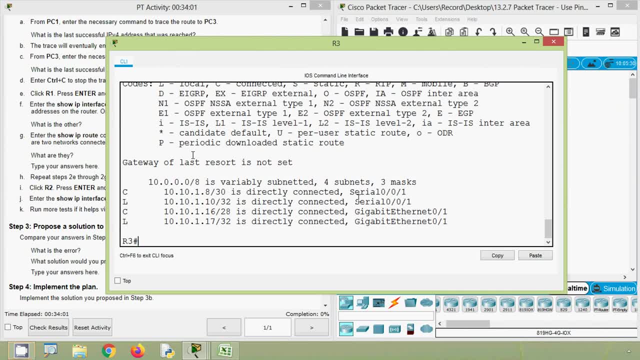 okay, now we will give show ip root. now, here we can see uh two networks are uh connected to this interface: serial zero, slash zero slash one connected. 10.10.1.8 slash 30 is directly connected to serial zero, slash, zero, slash one. then this local 10.10.1.10 32 is directly connected. serial zero. 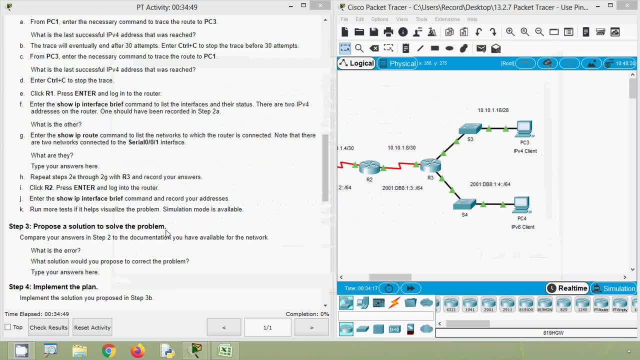 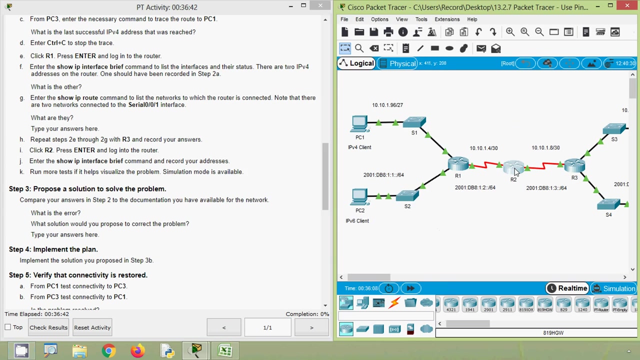 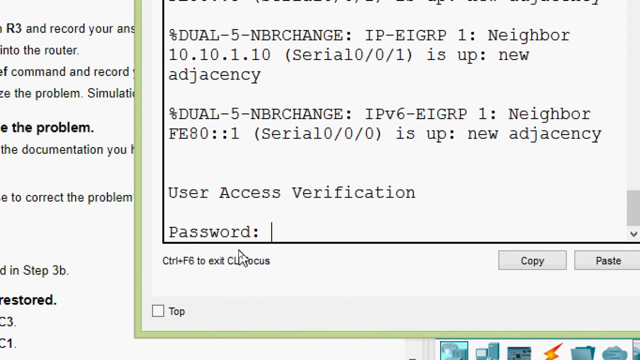 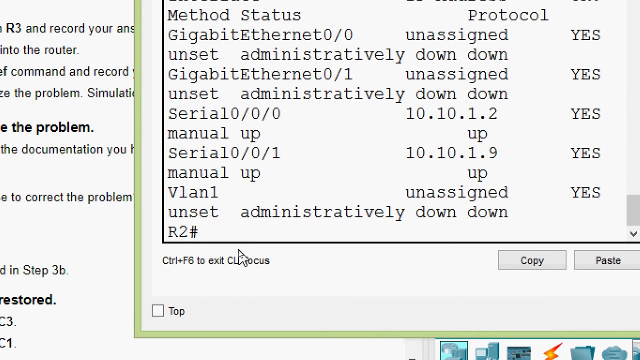 slash zero slash one outgoing target security. now click r2, then press enter and login to the router. enter the show ip interface brief command and record your addresses and more test. if it helps visualize the problem, simulation mode is available. Cisco enable password as class. show IP interface brief and we will verify its. 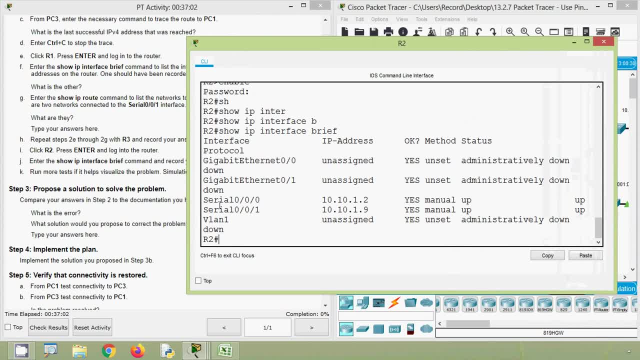 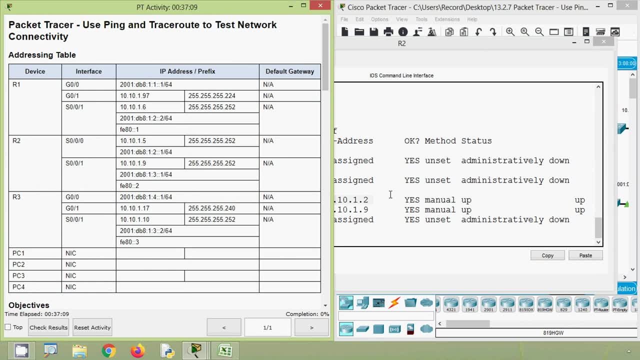 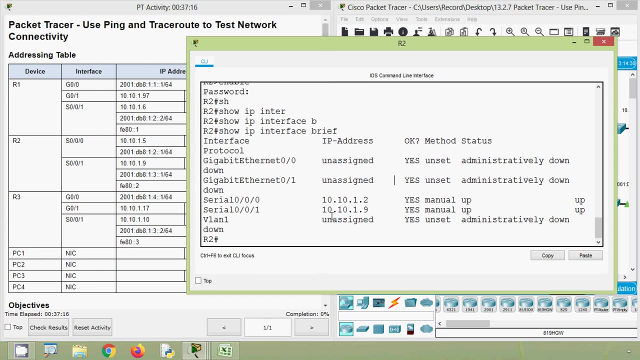 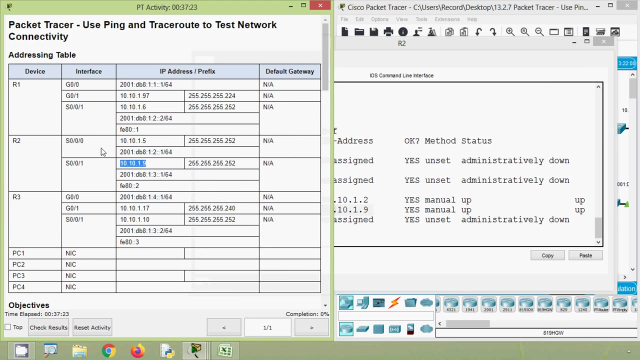 IP address: serial 0- slash 0, slash 0. 10 dot 10 dot 1 dot 2 on r2. so we can see 10 dot 10 dot, 1 dot 9. okay, and for the interface: serial 0- slash 0, slash 0 here. 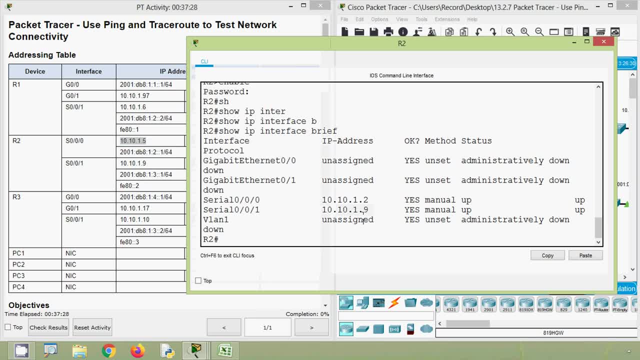 we can see IP address. it's a 10 dot 10 dot 1 dot 5, but it's given is a 10 dot 10 dot 1 dot 2. here the IP address for the interface: serial: 0, slash 0, slash 0. 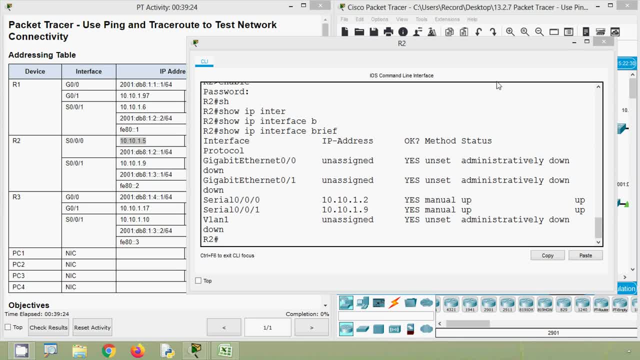 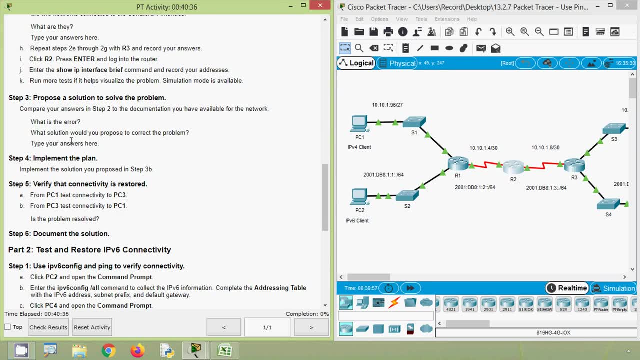 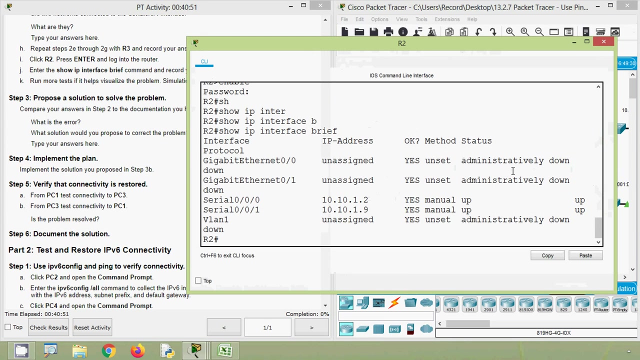 is configured incorrectly. okay, now, coming to step 3, propose a solution to solve the problem. compare your answers in step 2 to the documentation you have available for the network. what is the error? yes, already we have seen that in this router r2, configured the IP address for the interface serial: 0, slash 0, slash 0. 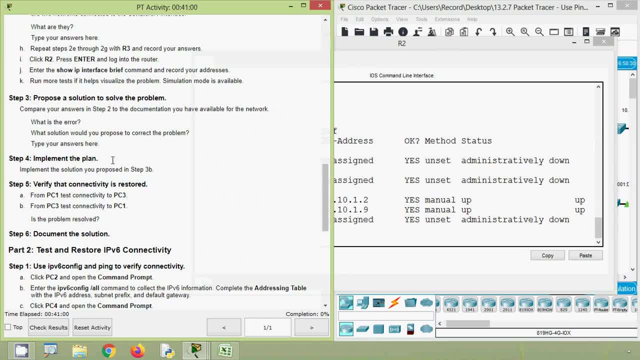 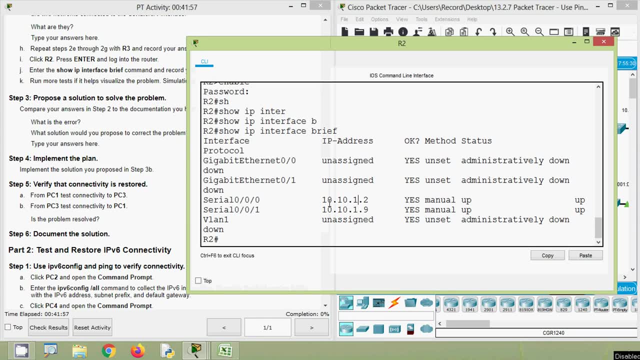 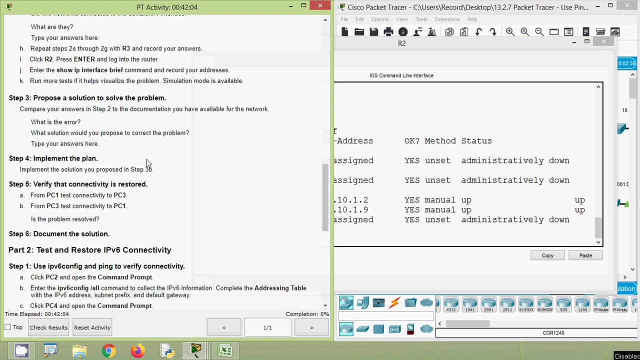 incorrectly. what solution would you propose to correct the problem? Obviously, we have to reassign IP address for the centrifuge, serial 0, slash 0, slash 0, as per our addressing table. Okay, now, coming to step 4, implement the plan. 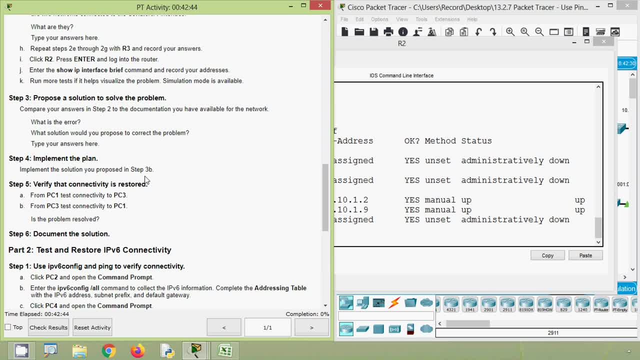 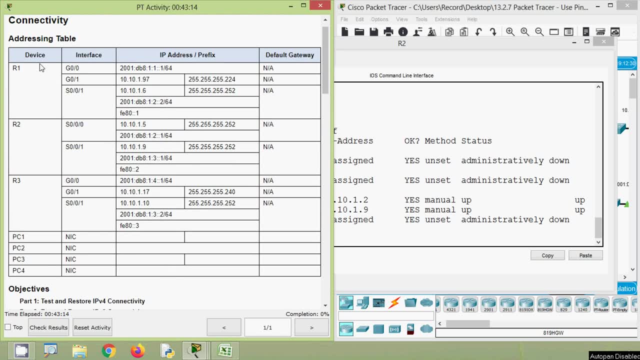 Implement the solution you proposed in step 3b. Okay, we will do that. We will copy its correct IP address from this addressing table. Here we can see that it's 10.10.1.5.. Also here we can see it's to mask. 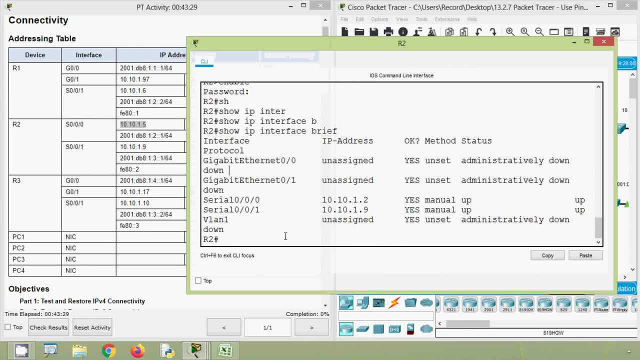 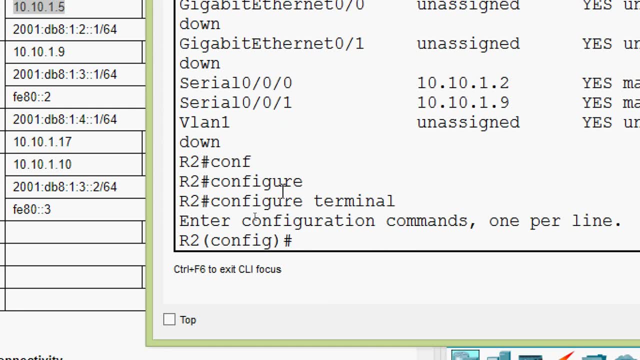 Okay, now, coming to router R2,. we will go to this interface: serial 0- slash 0, slash 0.. Configure terminal. we will go to the interface serial 0- slash 0, slash 0.. And we can assign this IP address: 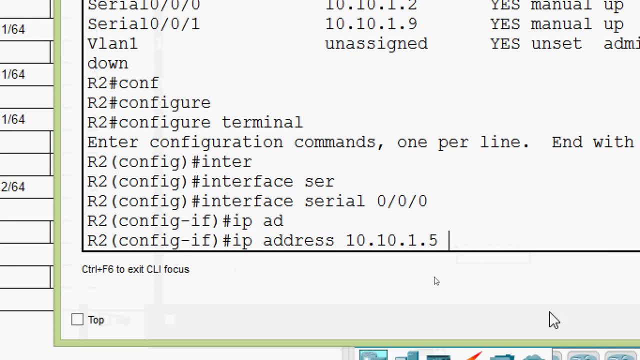 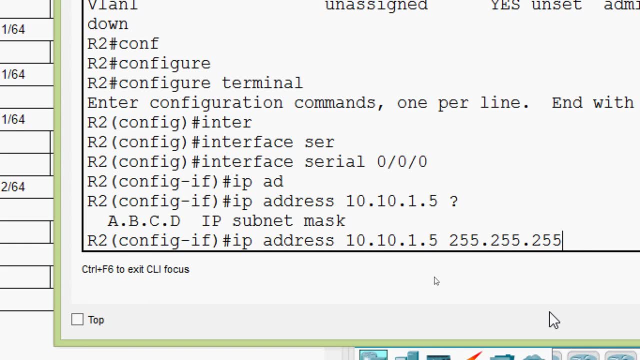 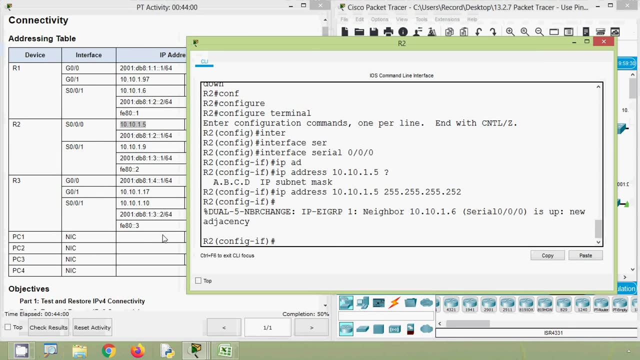 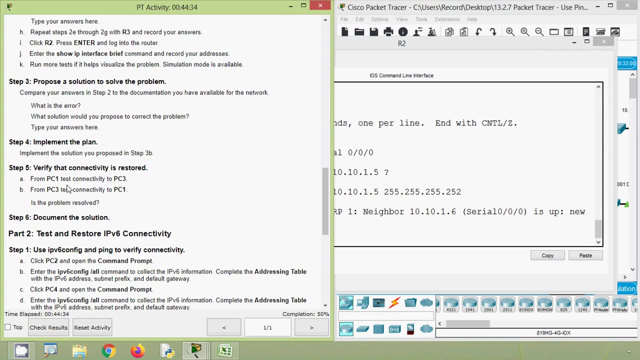 We already copied from our addressing table. Now we have to give its subnet mask. It's here. Then press enter Okay. Now in step 5, verify that connectivity is restored From PC1, test connectivity to PC3.. 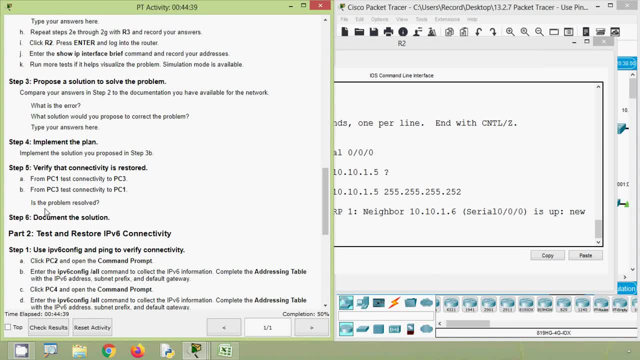 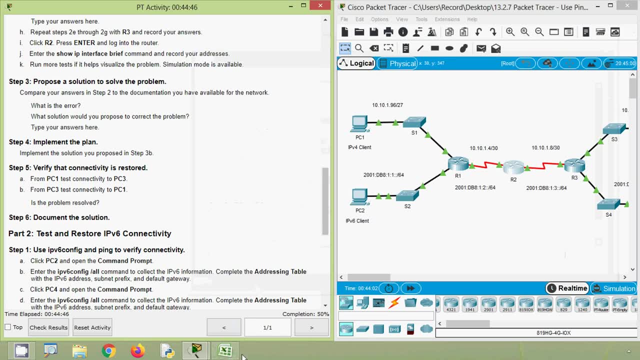 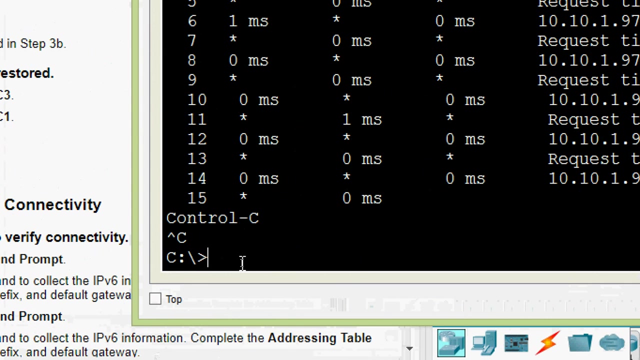 From PC3, test connectivity to PC1.. Is the problem resolved? Okay, we can try that. We will copy PC3 IP address. And coming to PC1, command prompt, Here we can use this up arrow, Yes, and here we can see the ping command. 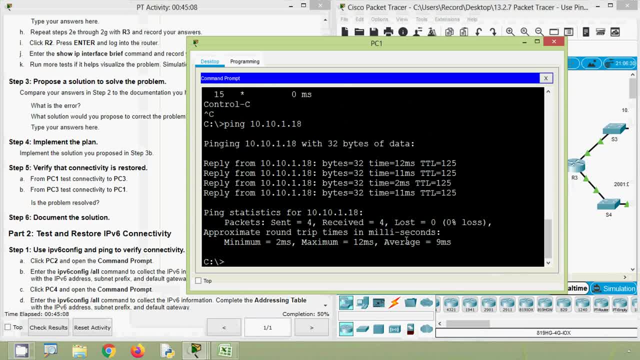 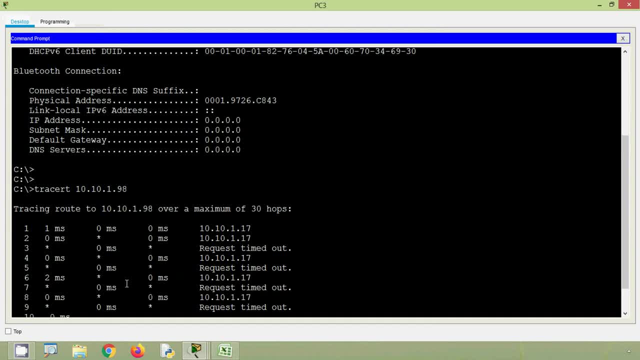 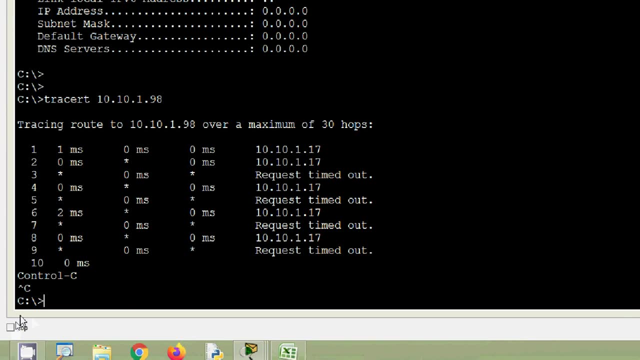 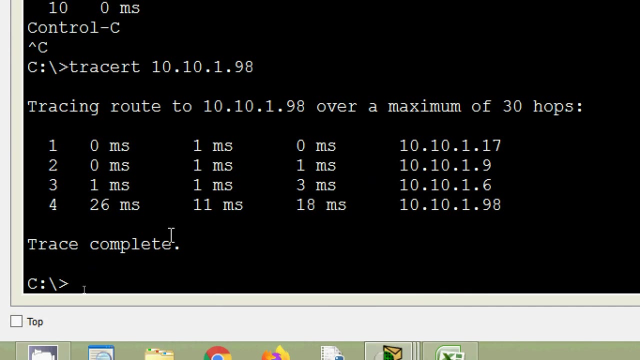 Then press enter. It's working. Now we will go to PC3 and we will ping to PC1.. Here also we can press up arrow so that we get that ping command. It's not there, Okay, So just we can give a tracer. 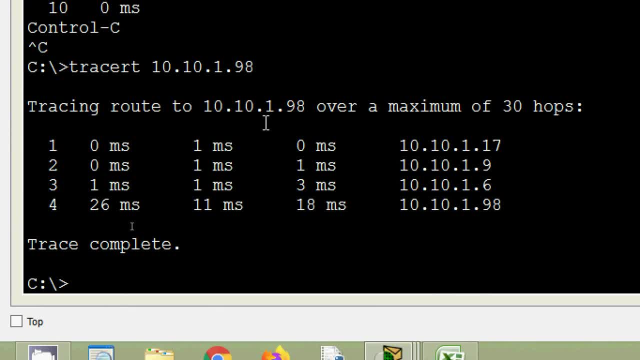 And here we can see trace complete. Even we can try with the ping. Okay, So instead of this tracer, we will give a ping. Instead of this tracer, too, we will give a ping, And here we can see it's working. 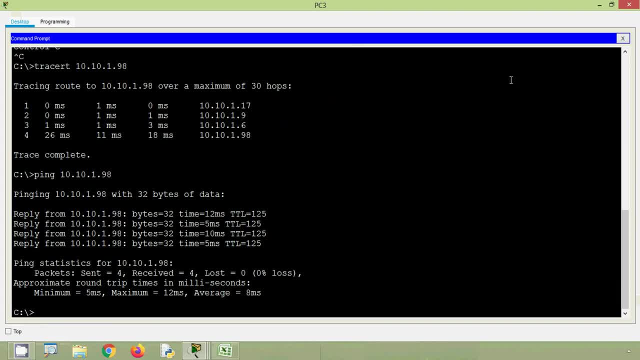 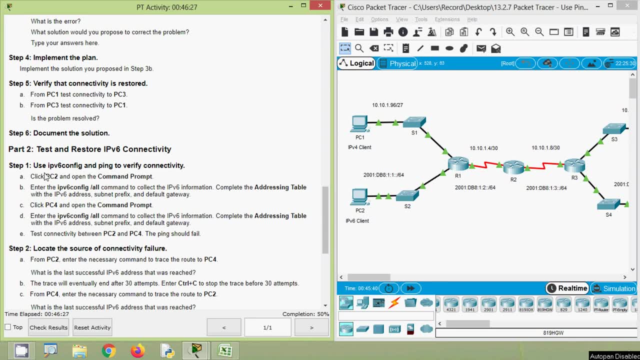 And here we can see it's working. Now coming to part two: Test and restore IPv6 connectivity. Use IPv6 config and ping to verify connectivity. Click PC2 and open the command prompt. Then enter ipv6 config space. slash all command to collect the IPv6 config. 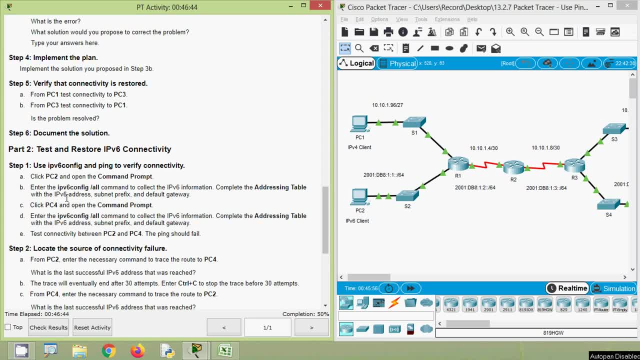 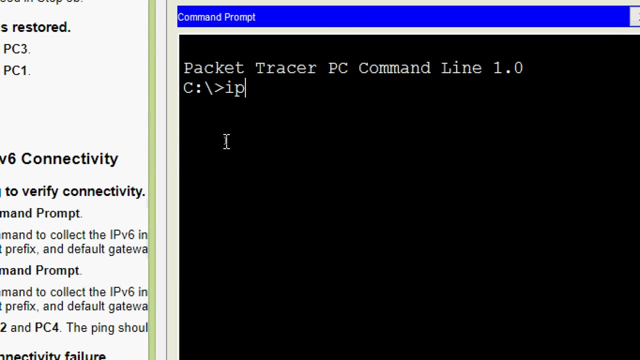 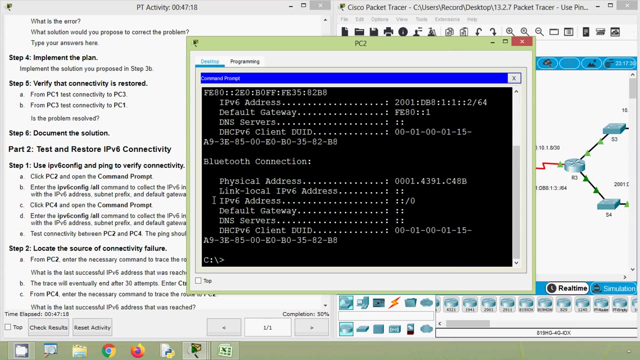 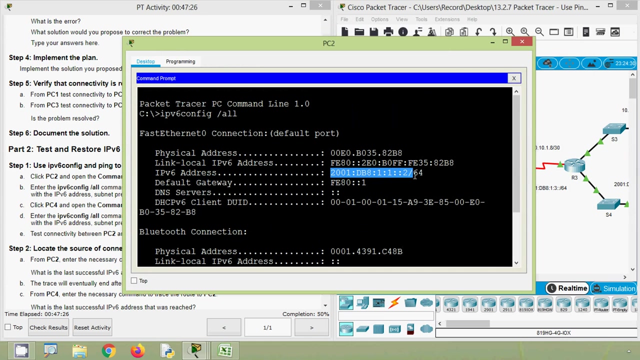 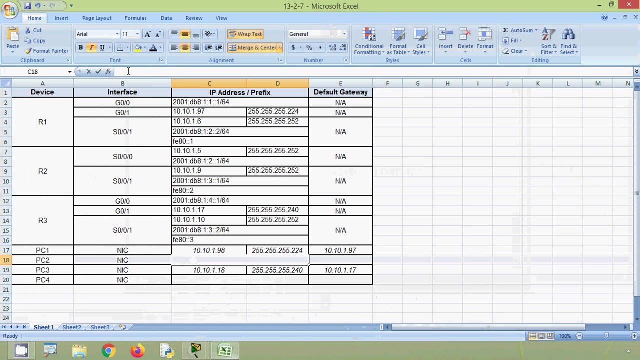 information. then complete the addressing table with the IPv6 address subnet prefix and it's a default gateway. we will go to pc2 command prompt. here we will give IPv6 config space, slash all, and here we can see it's IPv6 address. we will copy it and come into our spreadsheet pc2 and here is our IPv6. 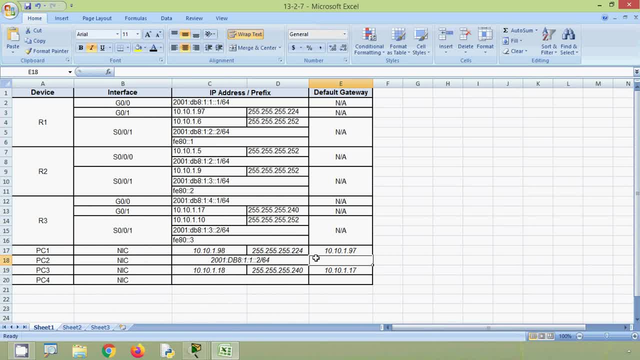 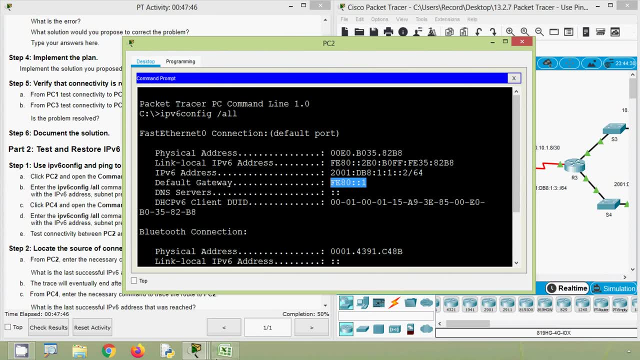 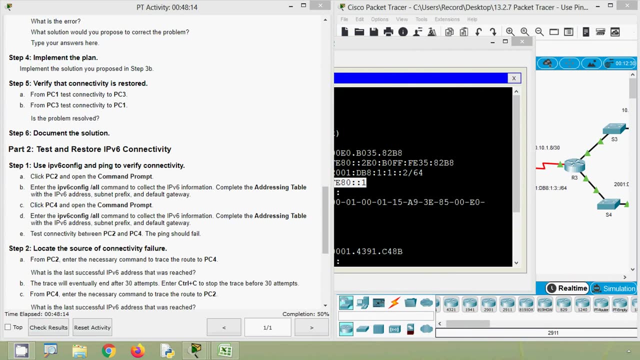 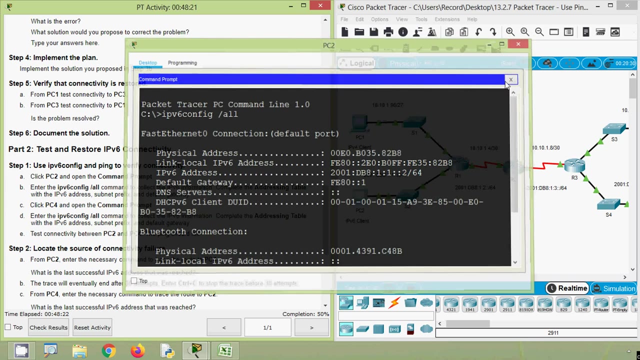 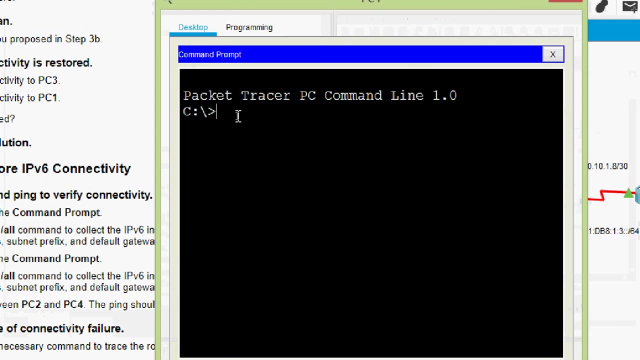 address. so with its a prefix, now it's a default gateway, you it's your. we will copy that right. in the same way we have to get from pc4 using its command prompt. okay, we can do that. we will go to pc4 command prompt. sure, we will give IPV6 config all. 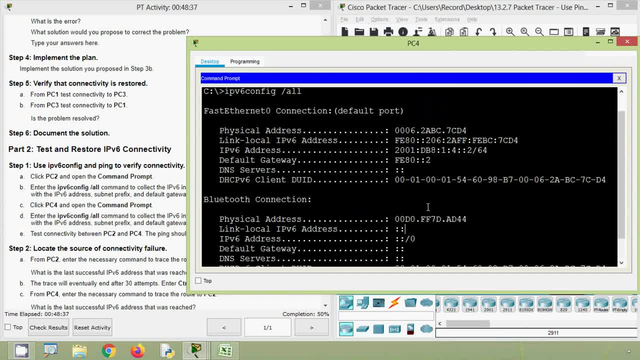 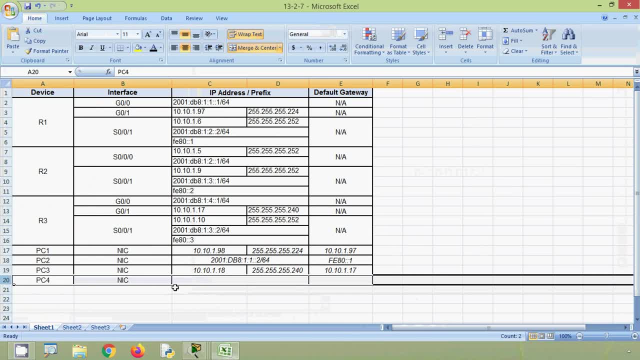 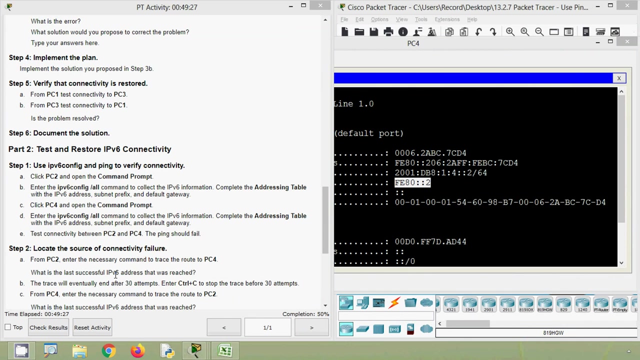 now we will check it's IP v6 address. it's your will copy that coming to our spreadsheet, PC for IP address prefix. okay, then it's a default gateway. it's your will copy that and it's your done here. okay, now test connectivity between PC 2 and PC, for the ping should fail. 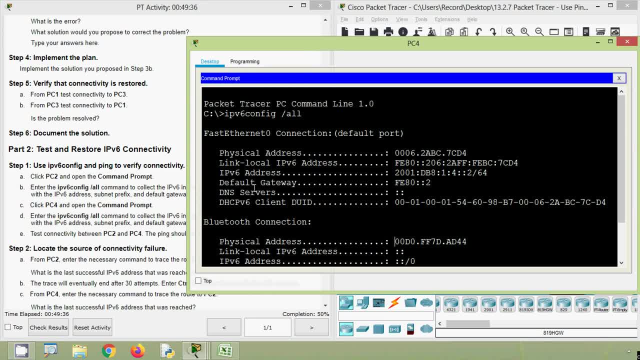 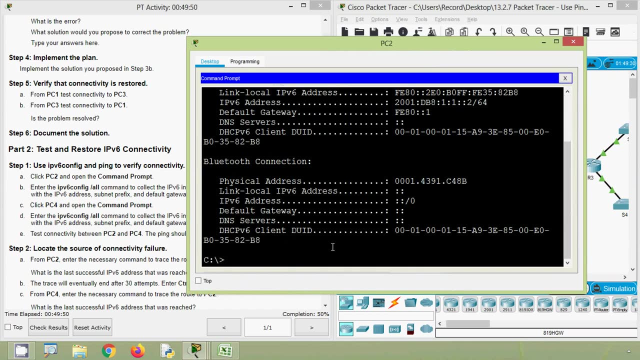 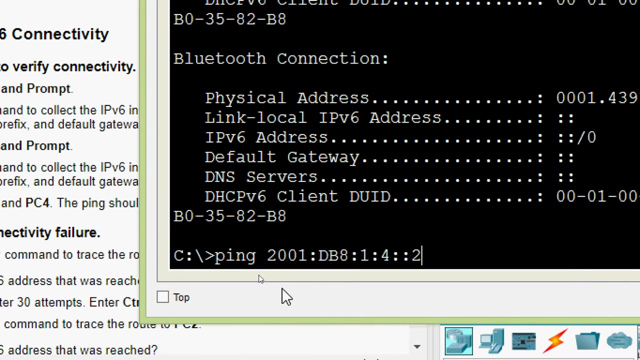 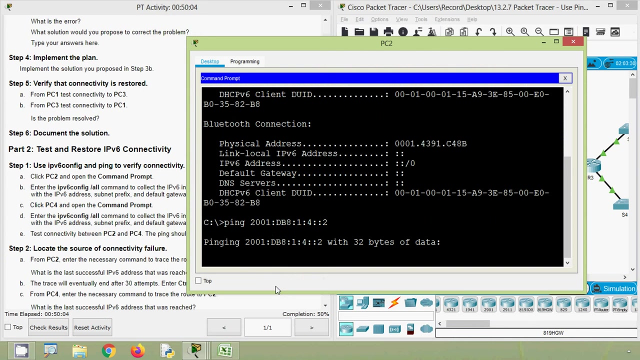 okay, we can do that. so here we will copy this apc for address and we will go to PC to command prompt and here we will give ping, then ipv6 address, the ipv6 address of our pc4, and we are waiting for the replies. request timed out. 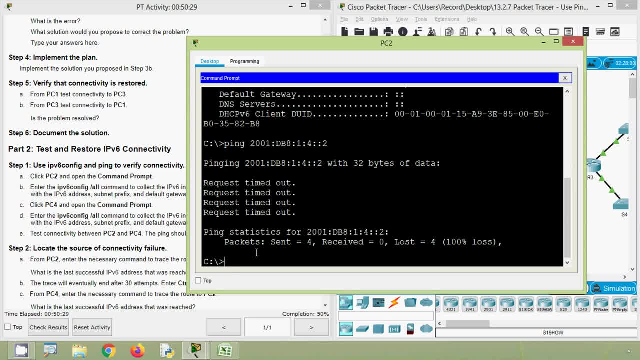 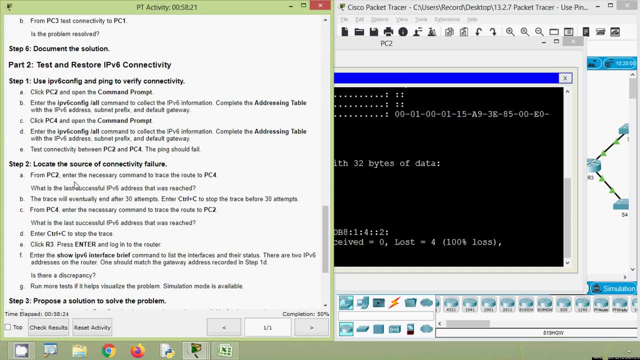 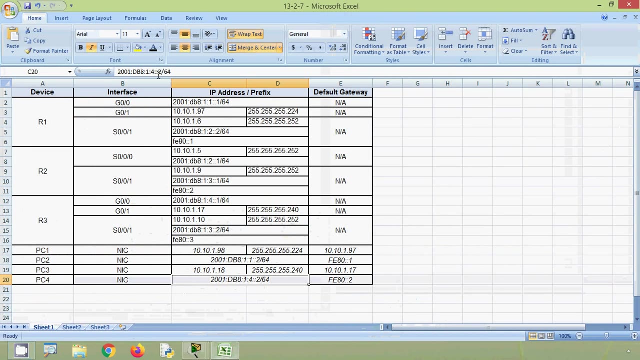 so here this ping failed. okay, now, coming to step two, locate the source of connectivity failure from pc2. enter the necessary command to trace the route to pc4. what is the last successful ipv6 address that was reached? okay, we will copy our pc4 ipv6 address. 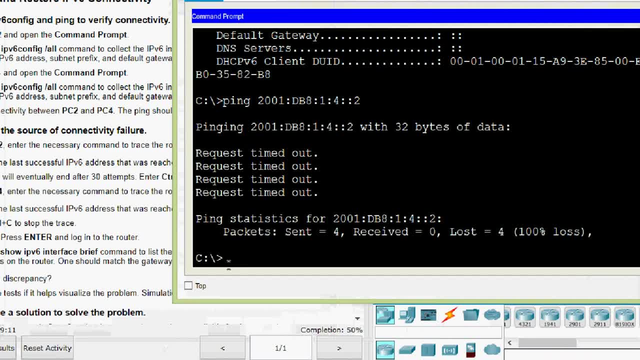 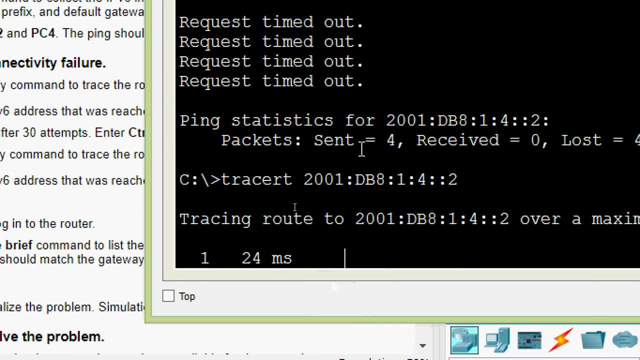 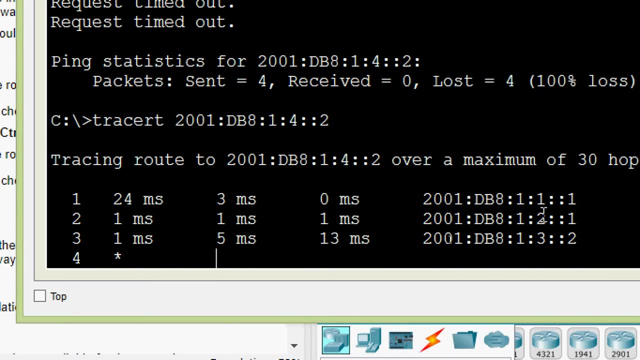 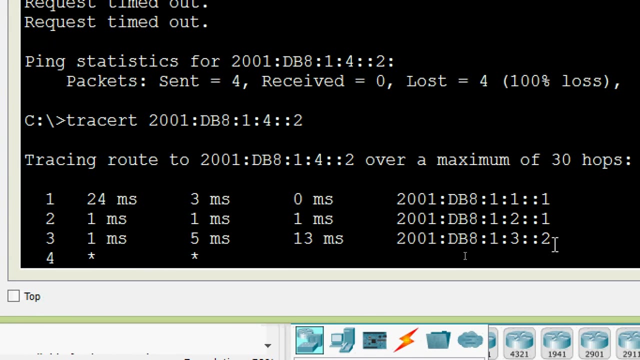 and coming to pc2 here, Here we will give a tracert, then our pc4 ipv6 address and here we can see it goes to 2001, colon tb8, colon 1, colon 1, double colon 1, 2, double colon 1, 3, double colon 2 and we 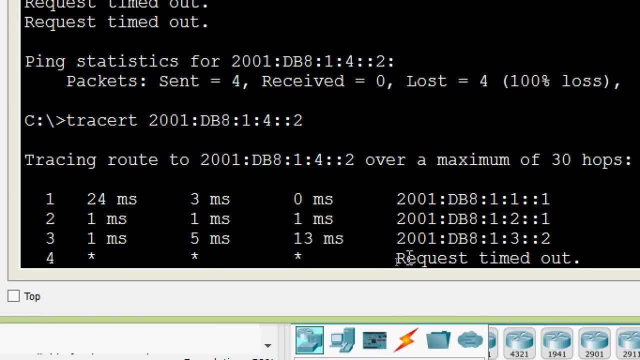 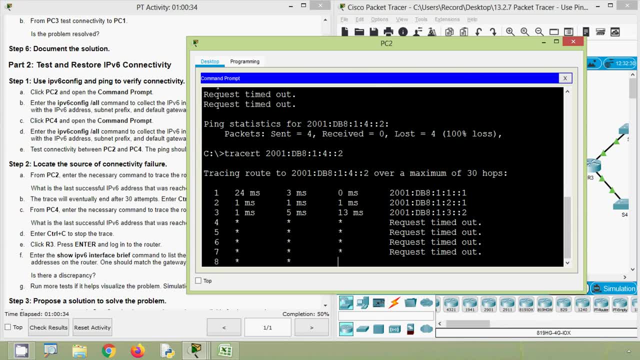 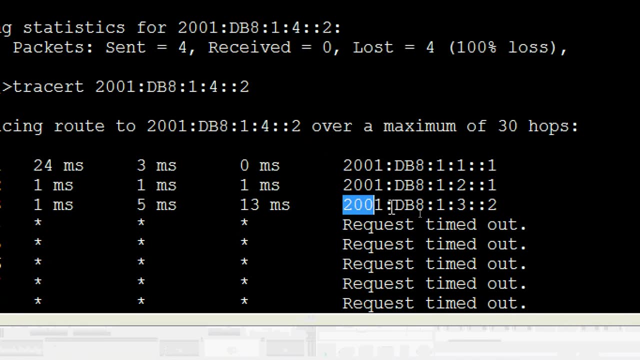 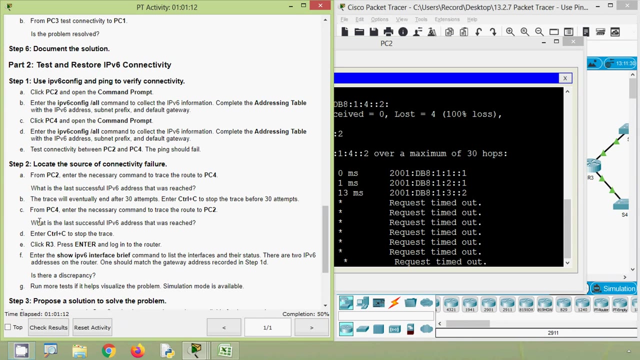 are waiting for the trace request timed out, and here we can see the last successful ipv6 address. it's a 2001 colon: gb8, colon 1, colon 3, double colon 2.. The trace will eventually end after 30 attempts Or enter control c. 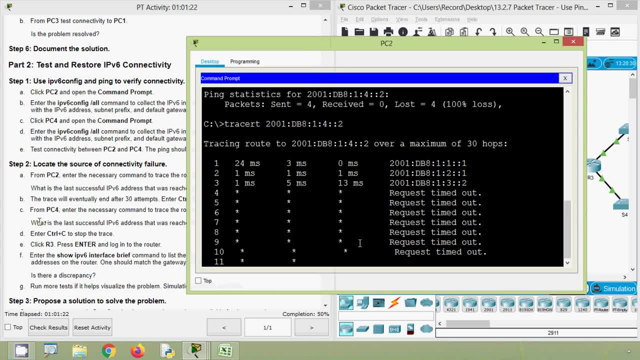 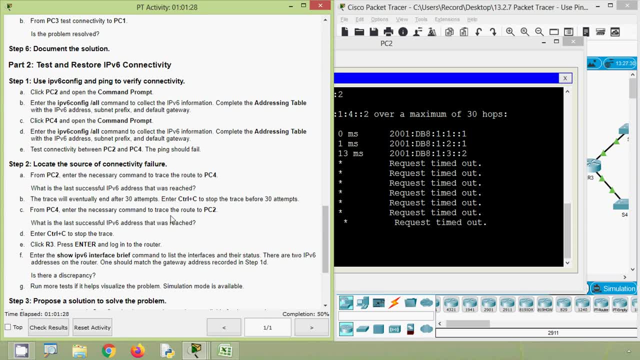 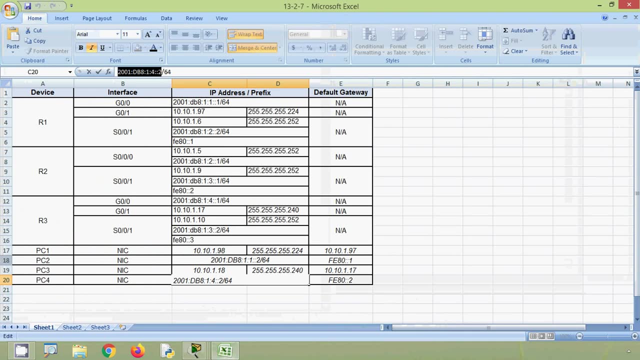 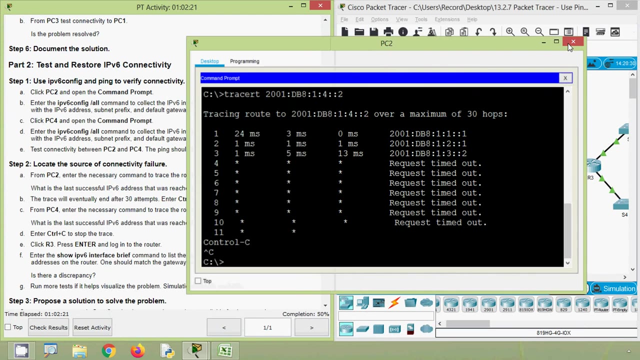 To stop the trace before 30 attempts. Ok, we can press control c Now from pc4, enter the necessary command to trace the route to pc2.. Now we will get our pc2 ipv6 address and close this pc2 and, coming to pc4, we will go to command. 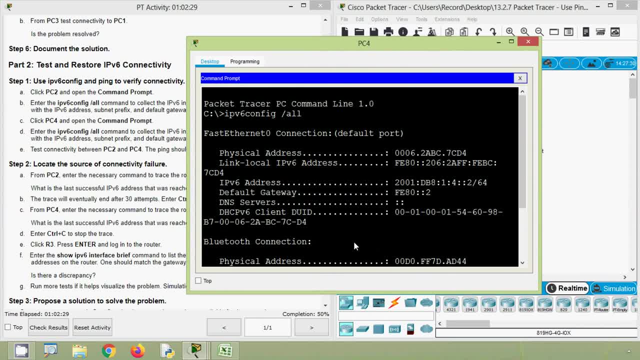 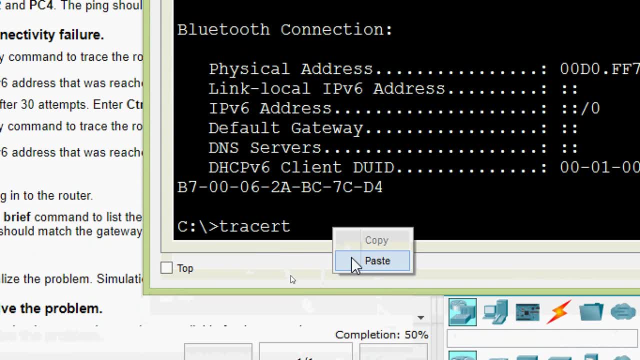 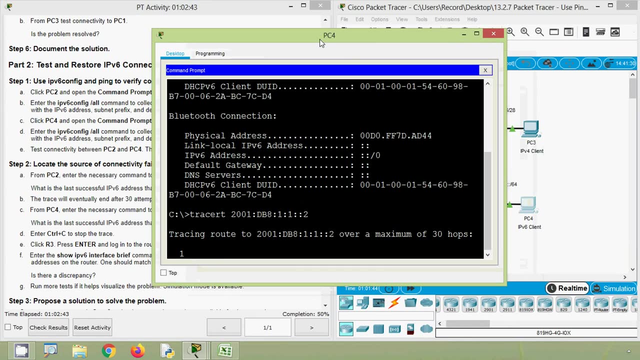 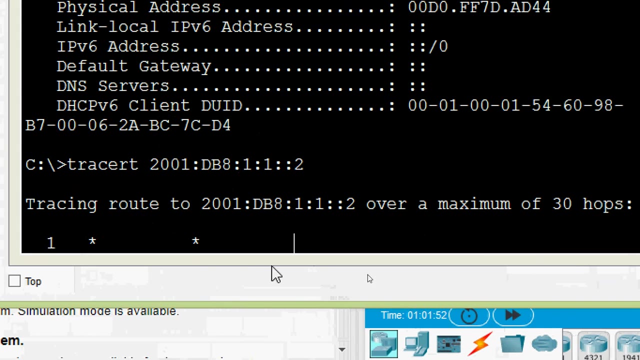 prompt And here we will give a tracert to pc2. here is our a pc2 ipv6 address And we are waiting for the trace. Click error. do not rrpf cannot flag. this is not our profess ox parameters. what it's like that 8.1 is sufficient. I'm going to close this check box here. 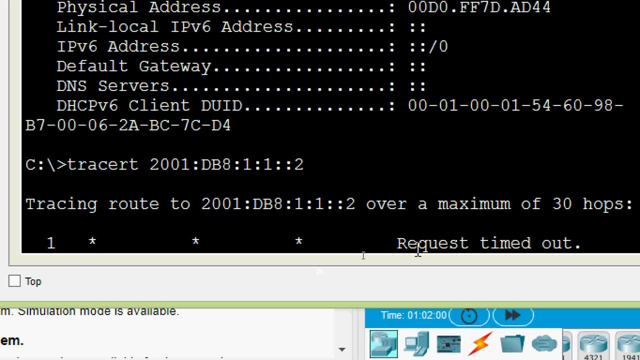 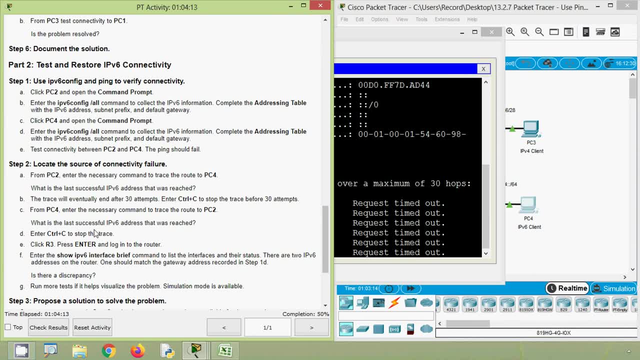 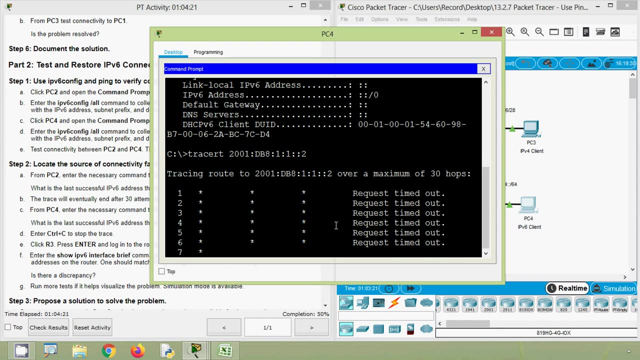 So Duplicate the versus trace and faster trace itself. we can see it shows a request timed out. now what is the last successful IP v6 address that was reached? so here in this trace we did not get any IP v6 address. so obviously I think the problem with the default 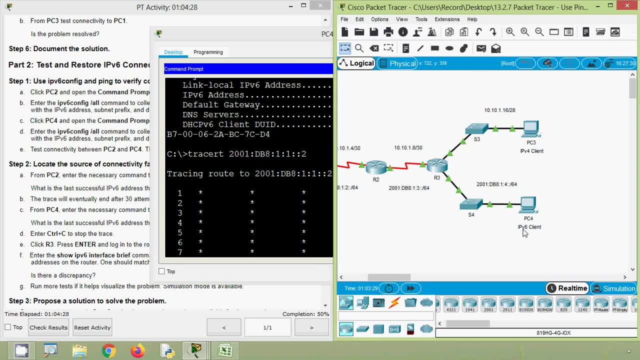 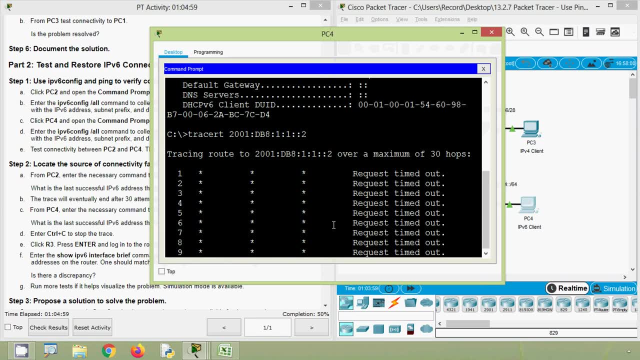 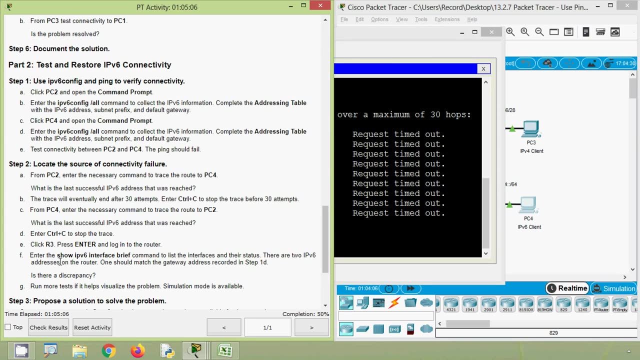 gateway in this device: pc4. okay, right, enter ctrl C to stop the trace. press ctrl C now, click r3, then press enter and login to the router. enter the show IP v6 interface brief command to list the interfaces and their status. there are two IP v6 address on the router. one should match the gateway address. 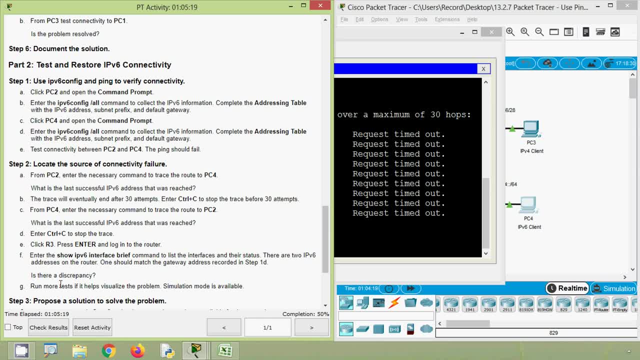 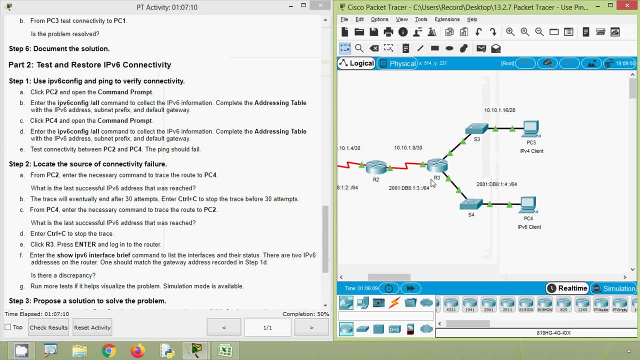 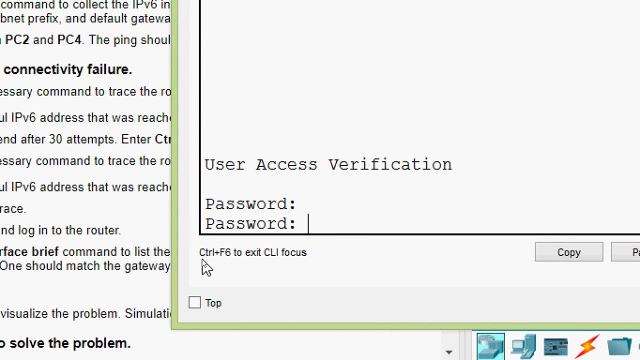 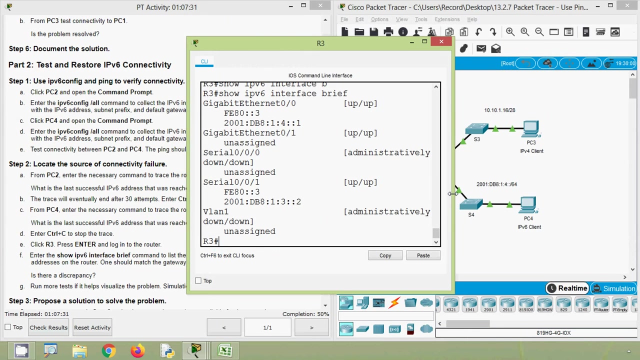 according step 1d. is there a discrepancy? okay, now we will close this pc4 and then we will go to r3. right password is Cisco enable password is class. here we will give a show. IP v6 interface- brief article pdf. now we will go to our. 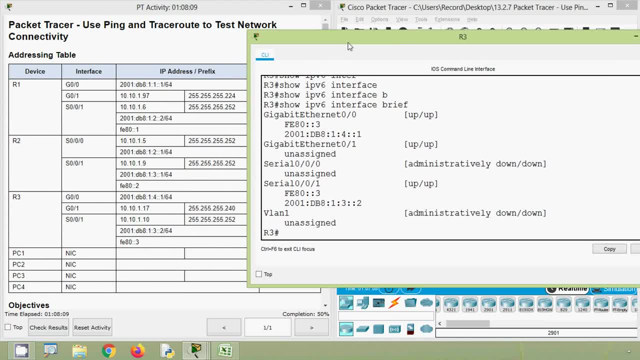 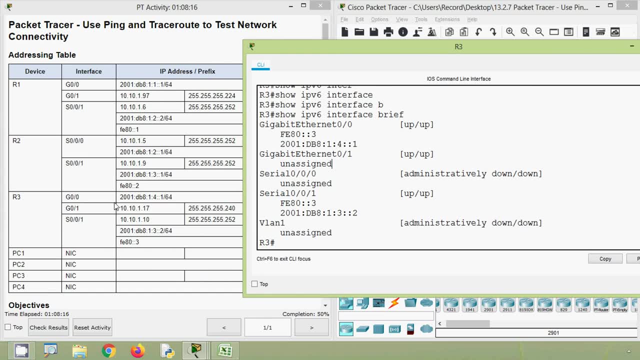 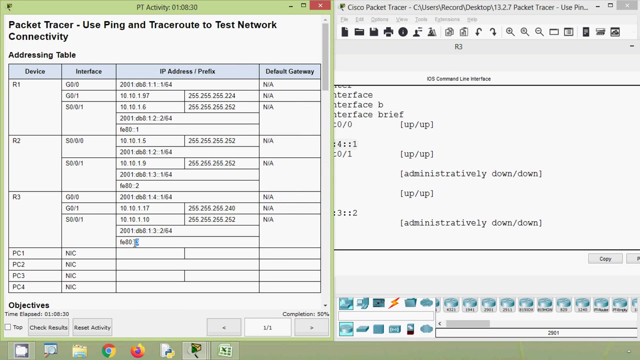 básiques, diffuser the archiving account and we will verify these addresses. so of course you can see the address of the router. No problem, we will create another address terminal. it's just fertilization. it's a good interface. now we will go to our addressing table and we will verify these addresses. so. 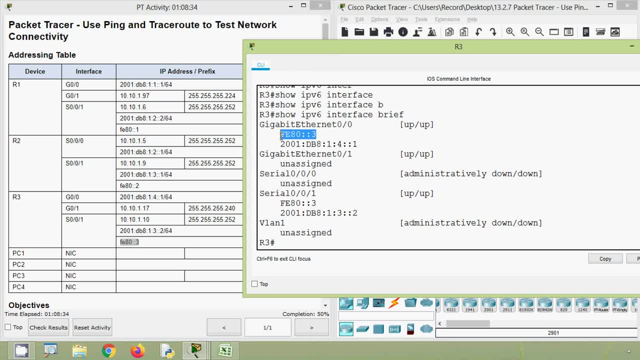 FE 80. double colon 3. and coming to serial 0, slash 0, slash 1: here we can see it's IPv6 address: 2 0 0, 1 colon TB 8. colon 1. colon 3. double colon 2: FE 80. 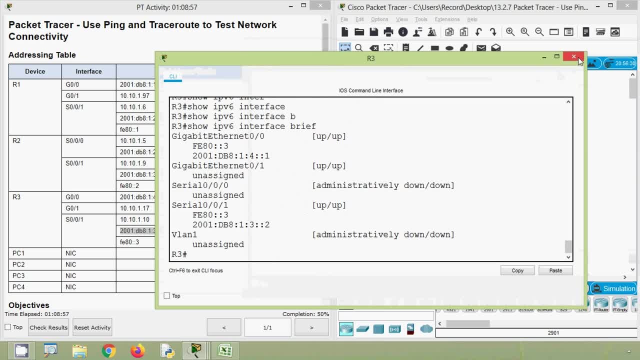 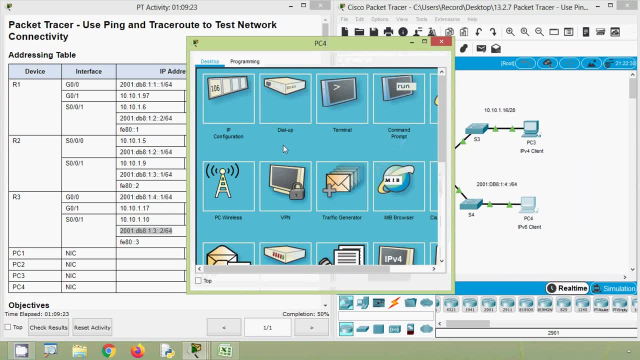 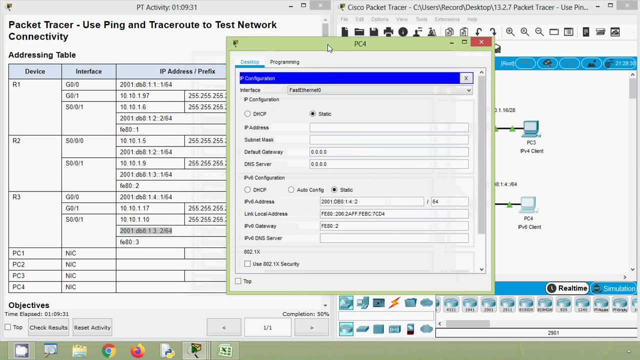 double colon 3. okay, it's correct. now we have a doubt with the PC for IP configuration. but I don't think so. it will go to- yes, it will go to- IP configuration. and here we can see it's IPv6 address and here we can see it's. 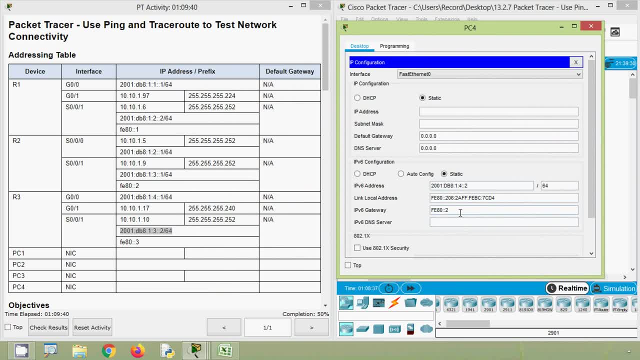 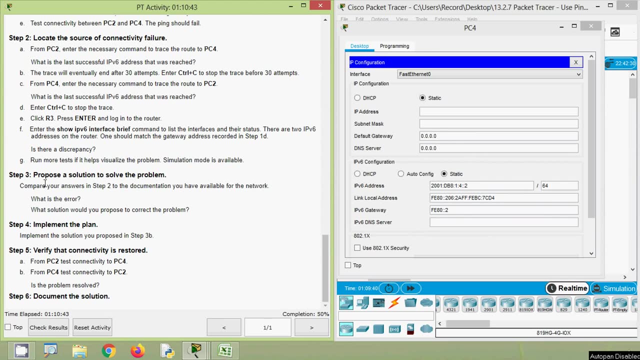 IPv6 gateway. here we can see this IPv6 gateway is configured to IPv6. and here we can see it's IPv6 gateway is configured to IPv6 incorrectly. it should be FE 80 double colon 3, but here they configured FE 80 double colon 2. now, in step 3, a proposed a solution to solve the problem. compare: 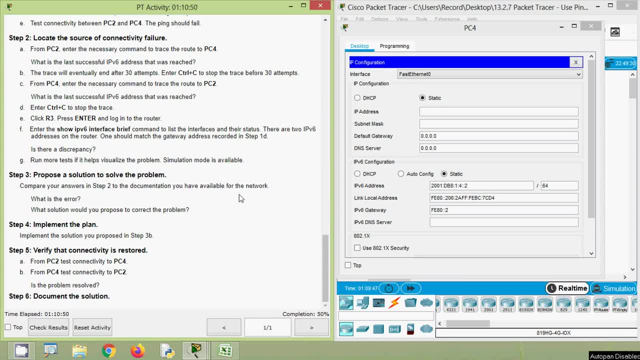 your answers in step 2 to the documentation you have available for the network. what is the error? yes, we identified it here. this IPv6 gateway is configured incorrectly in this device, PC. for what solution would you propose to correct the problem? we have to assign correct IPv6 gateway. implement the plan. implement the solution you proposed in. 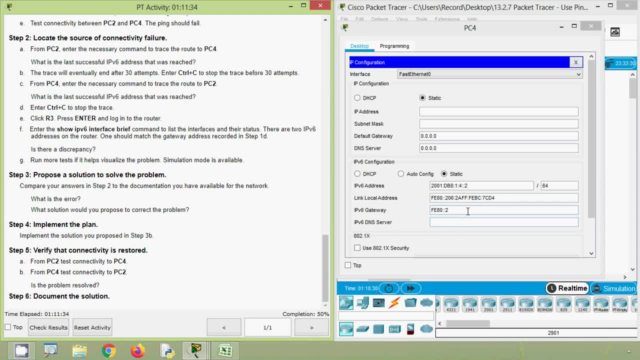 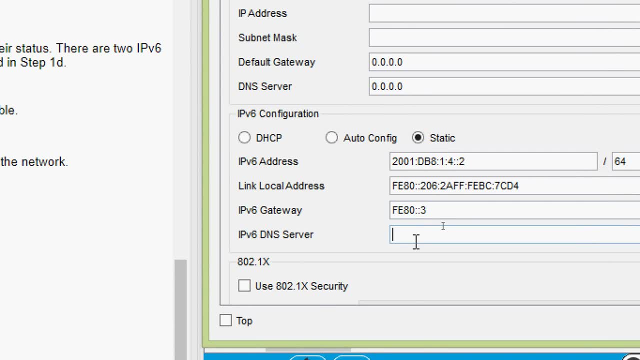 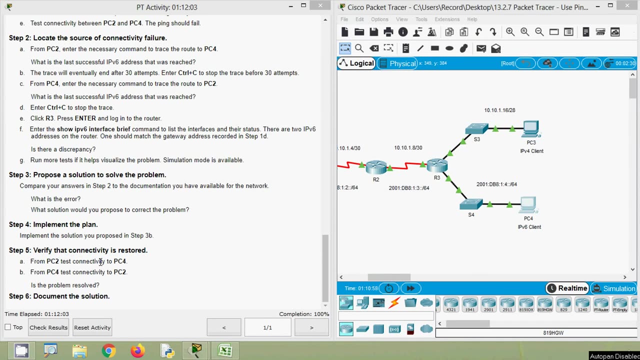 step 3 B. okay, here we have to change this IPv6 gateway to FE 80 double, colon 3. now, coming to step 5, verify that the connectivity is restored From PC2 test connectivity to PC4.. Then from PC4 test connectivity to PC2.. Is the problem resolved? We will verify that. We will go.